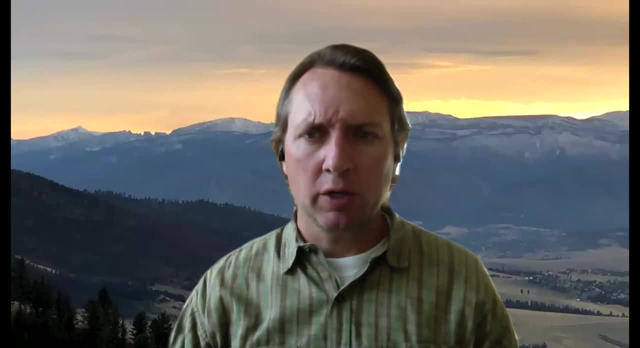 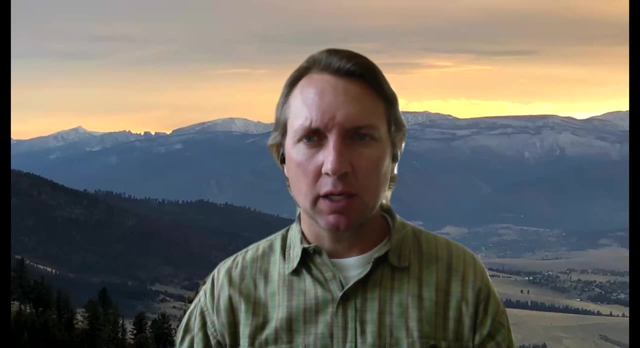 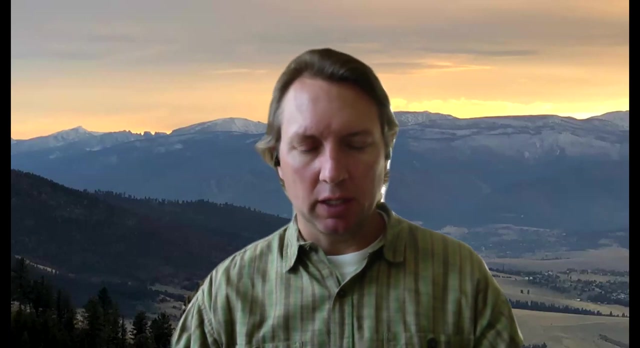 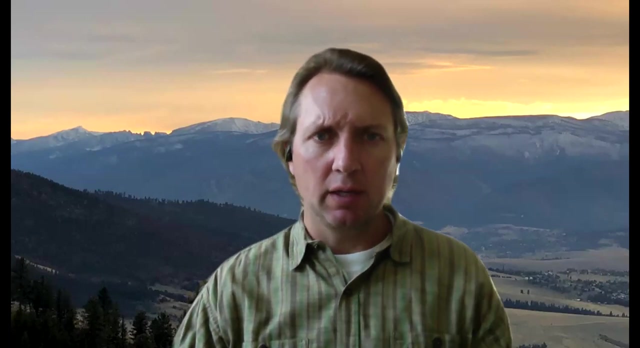 Hello and welcome back to GEO 420,- sorry, GEO 572, Advanced Hydrogeology. We're going to continue our discussion of conceptual models and conceptual model building. So, if you recall, when we left off last time, we had talked about what a conceptual model is, what 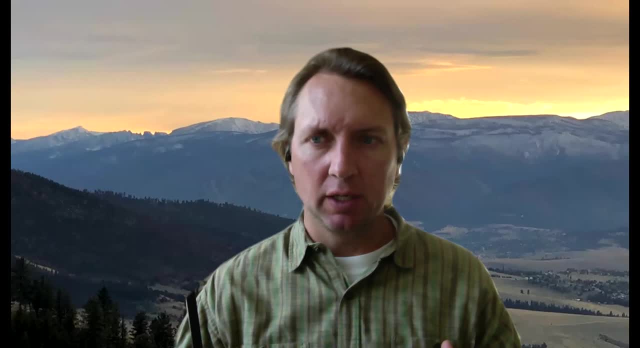 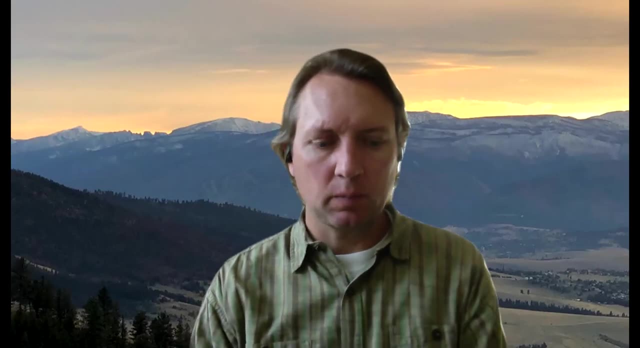 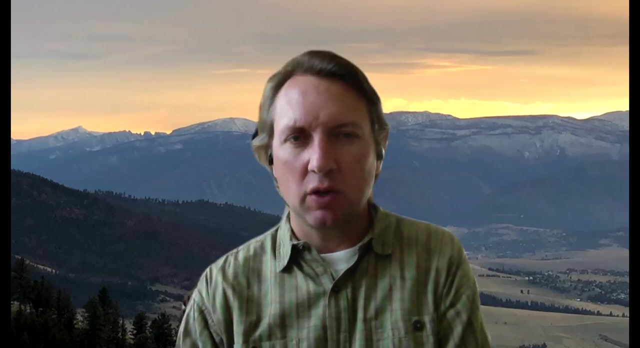 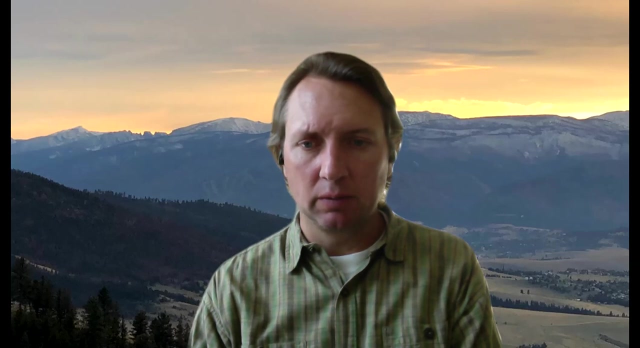 it entails. and basically, we decided that the conceptual model is a summary and a cartoon that contains all the necessary ingredients for us to solve the boundary value problem or to create a groundwater model. So today, what I wanted to do is talk about an example. 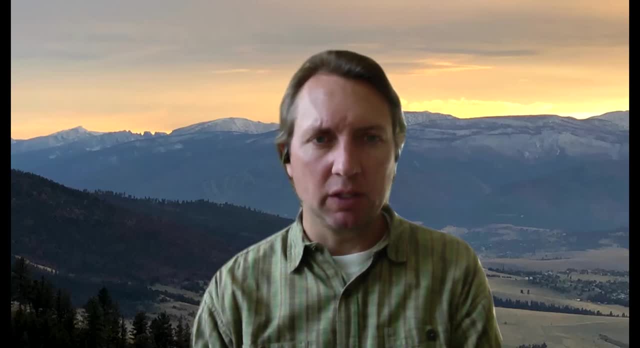 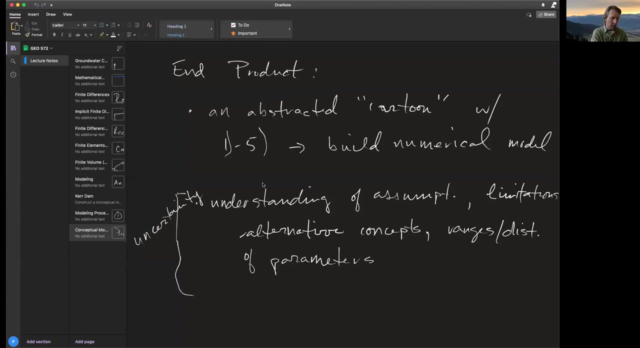 where we might think about some of these: how to build a conceptual model and how we go about starting to build that. So let me share my screen here. Okay, so here is where we ended yesterday, or the last lecture, and we said that the end product of this conceptual 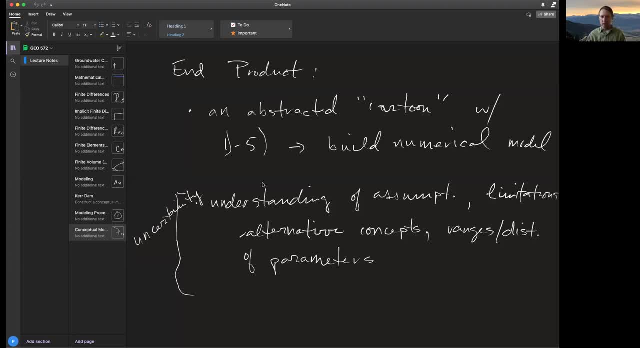 modeling exercise is an abstracted cartoon. All right, cool. So this is an abstracted cartoon- quote unquote- which contains all the ingredients needed to construct or to solve the boundary value problem And from that we're going to build the numerical model And remember as a caveat during this construction process. 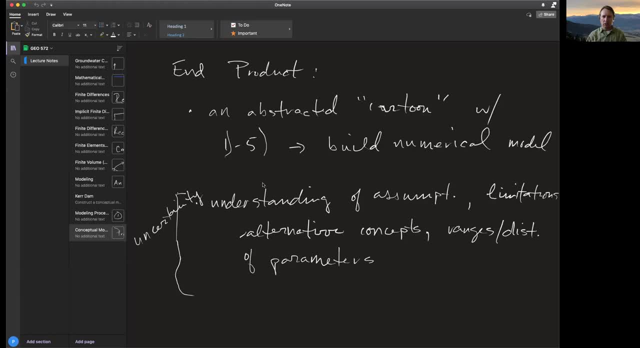 we're trying to make sure that we continue to think about uncertainty and understanding how assumptions and limitations and alternative conceptualizations might affect our modeling process. So let's go and talk about an example to give some concrete advice or concrete evidence of how we might build one of these conceptual models. Okay, So we're going to actually start. 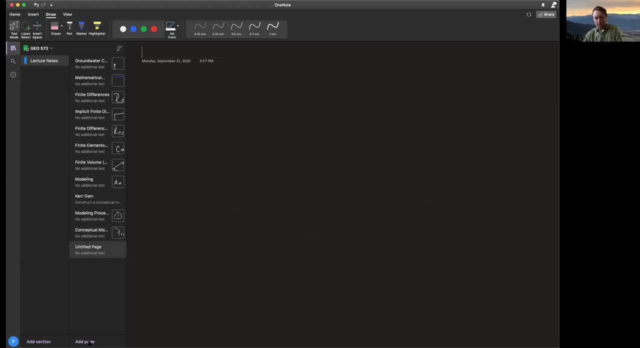 off with a problem that is very current. This is a problem that the Montana Bureau of Mines and Geology is working on right now, just outside Missoula of Lolo Creek drainage, And so this is the Lolo Creek conceptual model. Okay so, 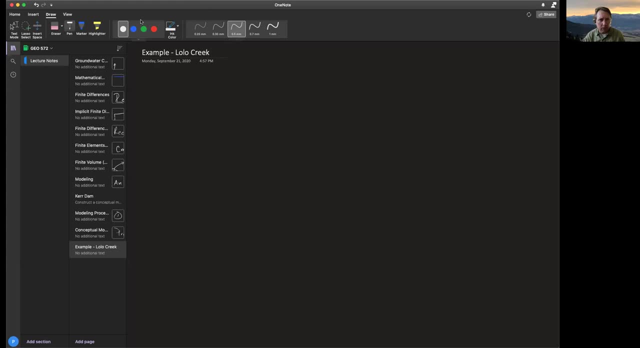 here's the idea I'm going to try and draw in map view an overhead of sort of Missoula Valley. and and Lolo, Here is a one mountain block on the north side of the Missoula Valley. This is the Rattlesnakes Rattlesnake Range. We got the Hell Gate All right. here is the. 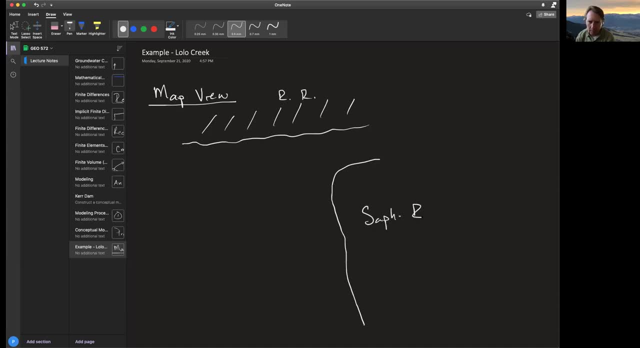 Sapphire. Down here we've got the northern Thinner Root Range, And then here this is the northern Thinner Root, And here below it is the Thinner Root range. All right, so in here we've got the Clark Fork flowing through the Missoula. 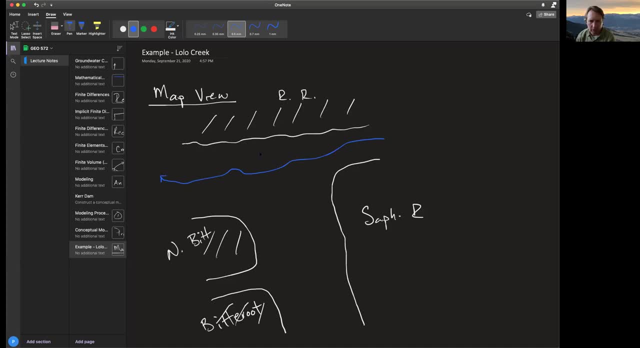 Valley and out towards Crenchtown. So here's the Clair Fork And then here the down this valley. we've got the Bitterroot River flowing into the Clark Fork. here we've got Lolo Creek coming out of the mountain block all right out into the Bitterroot Valley and joining the Bitterroot River. 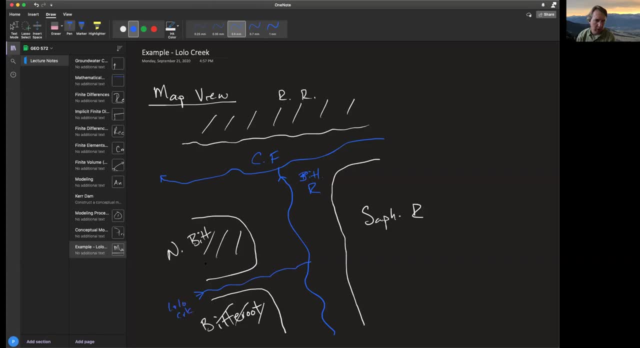 Lolo Creek and we have the town of Lolo. it sits right here at the mouth, all right near the intersection of these two. there's Lolo, and one of the things that's happening in Lolo's expanding and they're installing a new groundwater. well, let's say this: dot marks location, groundwater. 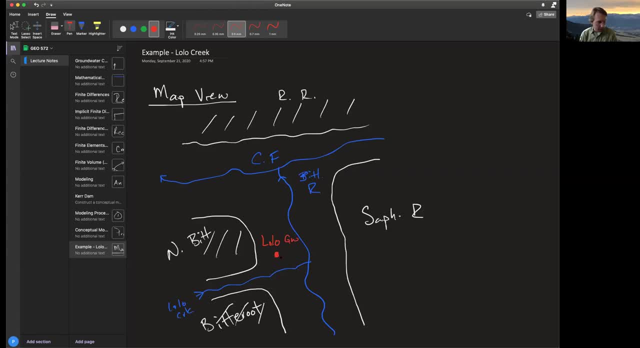 well, and a big concern right now is, as as they pump more and more groundwater out of this municipal well, how much stream water does Lolo Creek or how much of Lolo Creek stream water does this well intersect? so the question here: how much stream water does Lolo Creek intercept? sorry, does Lolo municipal well intercept? 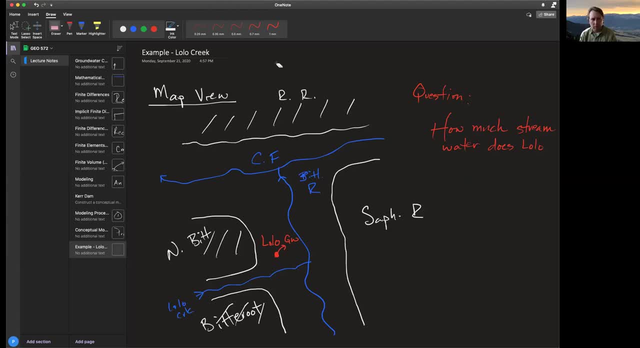 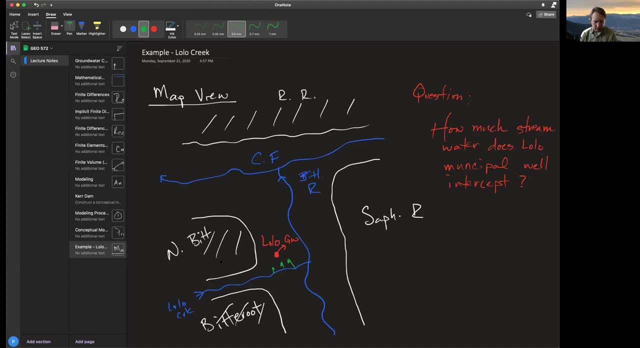 a cross section. here it goes: mountain range, cross the well into the sapphire range. get this cross section line we're going to draw as a a prime, all right. so let's also look at what this will make. a drawing here the of what this looks like in cross-section view. So here's map view. Let's look at it in cross-section view. 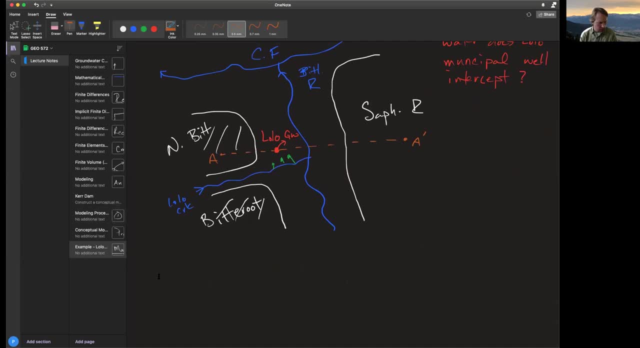 Cross-section A to A prime, All right, and we're going to just draw a generic cross-section here. So we start off in the mountains, All right, so we're up here in the mountains, Mountain block comes down, Comes out into the valley. 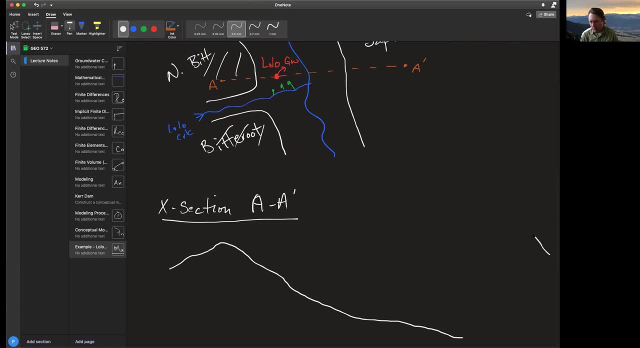 And then on the other side there's another mountain block Comes up and it comes down. We've got these two mountain blocks. I'll throw on a little bit of stratigraphy here, Just because I like to think about it. So here's A. 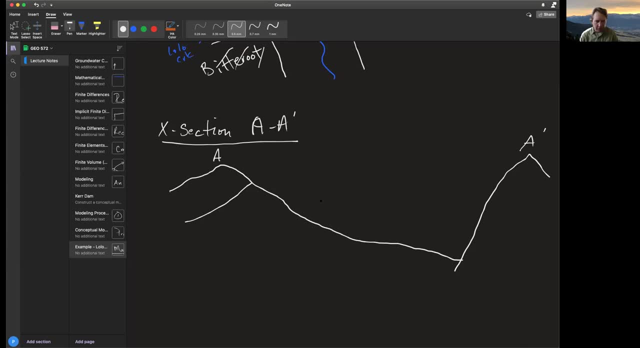 This is A prime Some stratigraphy of the Missoula group. Bonner Formation, Mount Shields. We've got the Shepherd Snow Slip And beneath that is the Wallace, And here we're on the sapphires. We're back in the same. 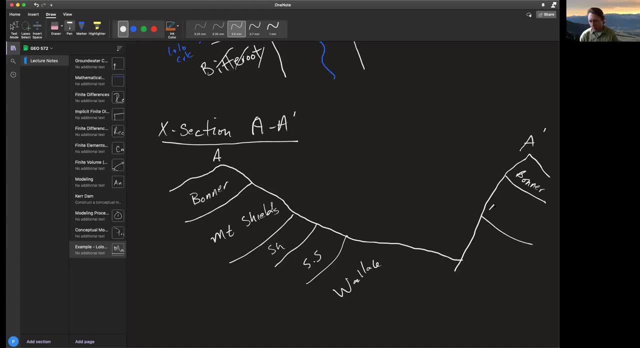 Stuffs of Bonner, Mount Shields, Shepherd, Snow, Slip, Wallace. All right, this is not perfect cross-section, But it gives you some idea. We're in the belt rocks. This is all the belts. All right, same as over here. 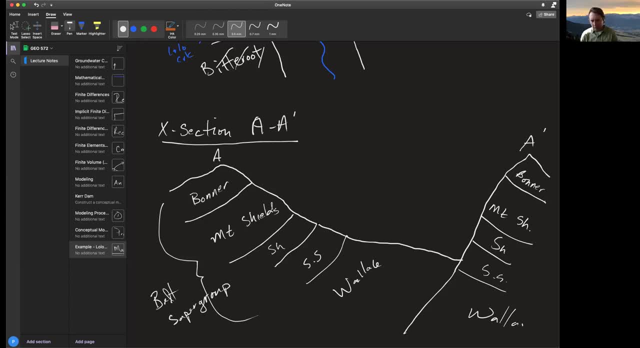 Our valley, however, is full of sediment. Here's the valley. I'm going to put a bit of a river in Here, Our low, low. well, All right, Here's the town of Lolo. Okay, The stratigraphy in here. So we've got a. 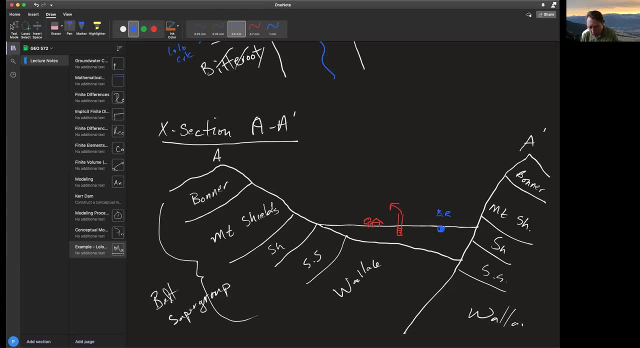 This is a unconvincing pond aquifer that goes to the river And this cartography in here. well, there's a bunch of gravels, some clay lenses in here, about 30 meters or so. that are more or less. 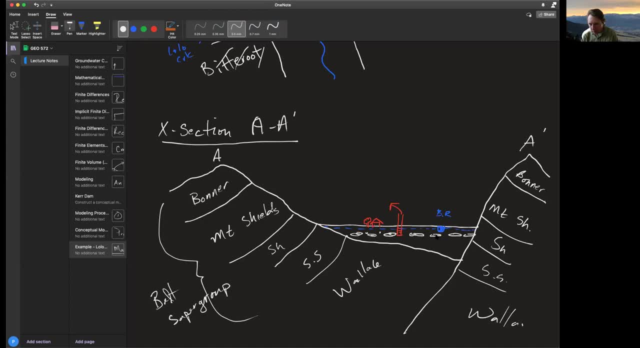 continuous, And up here it's sand and gravels And then beneath that we've got fine-grained sediments of theosine and myosine and fine-grained sediments. Okay, so this is a general conceptual model of what the geology looks like in the area. 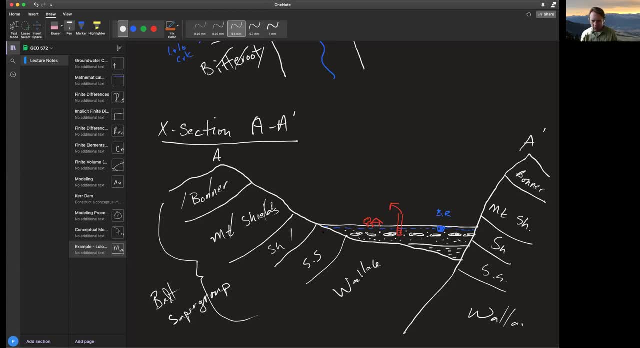 These are all fractured bedrock, mountain blocks and this alluvial aquifer that has a water table that's highly connectable to Volo Creek, And there's an upper aquifer in the sands and gravels that's really highly permeable. This is the upper aquifer. 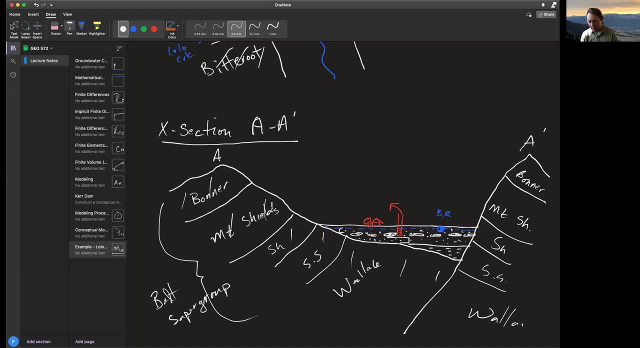 there's a lower aquifer. that's kind of a semi-confined aquifer beneath these more clay rich layers, so yields pretty well, but it's kind of disconnected from the river and down beneath that is a pretty low permeability unit. it's called the renova of fine grain myosin sediments. okay, so these are our two sort of first. 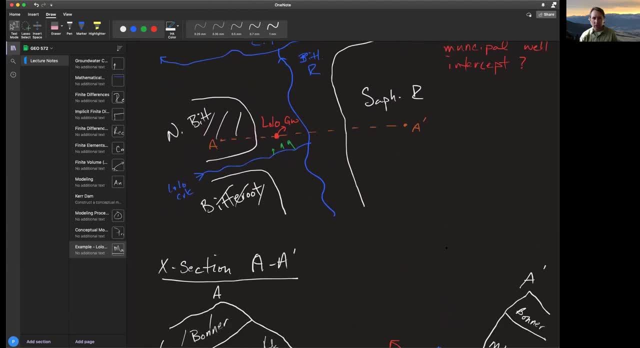 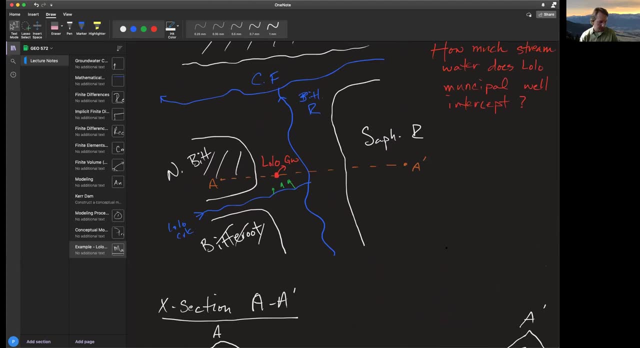 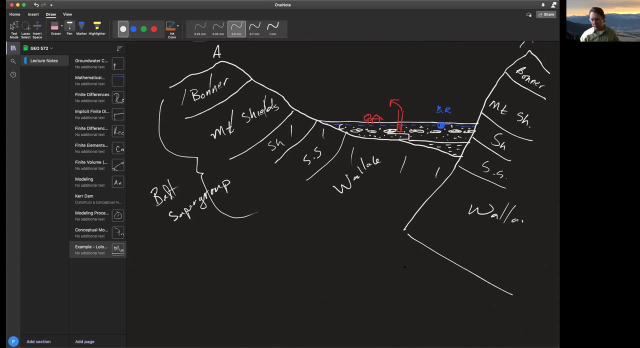 conceptualizations of geology, and what I want to start to do is pull some of the ingredients for making a model out of them. and beneath the wallace, both locations- is a pre-cambrian bedrock granites, piscis, just to complete our section. 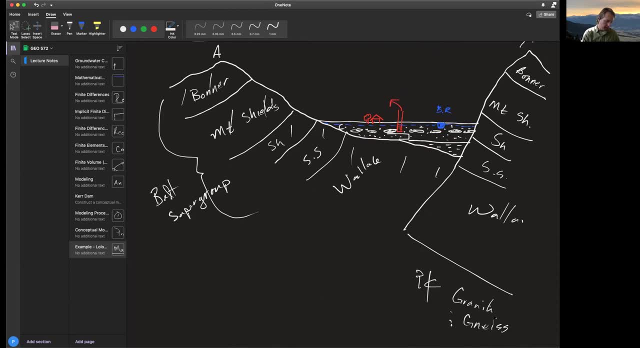 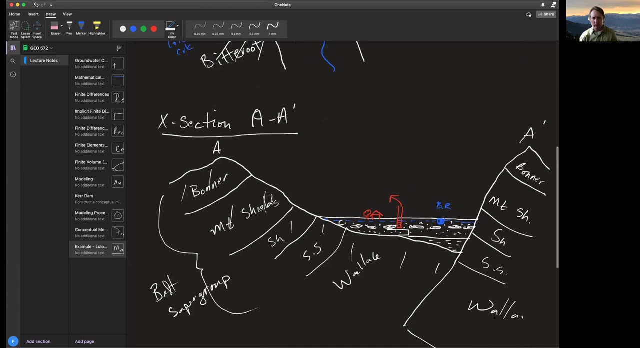 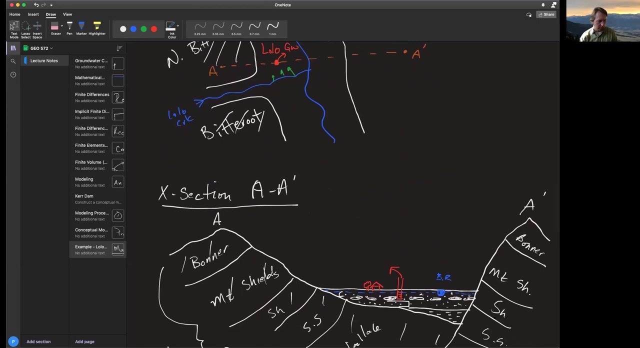 okay, let's, let's think about how we might start to think about making this guy into a model. so this is this is where the art of modeling comes in. when you've got this real-world situation, it's very complicated and we've got to start to abstract it. all right, and so the first thing we're going to recall is: 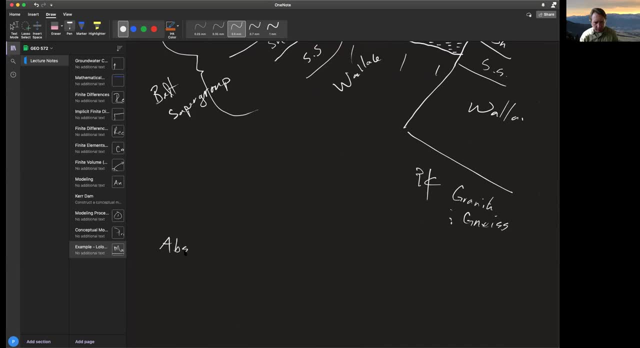 or remember that abstraction. it's the art of removing complexity while retaining salient features for answering our question. we want to retain the salient features. we want to retain the salient features. we're answering our question, you, you, but we want to remove complexity. So our job here is to 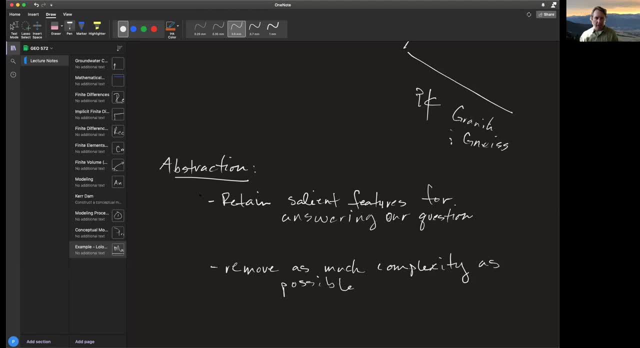 to do that and sort of a classic saying. I don't know what abstraction is or what a classic saying here is in the physics world is: Consider the sphere of a cow, All right, and basically there might be some times where considering a cow as a sphere 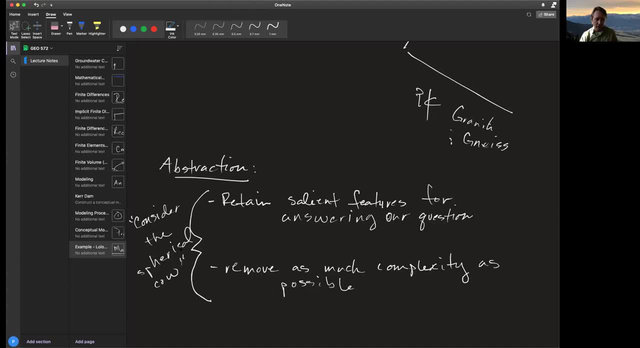 might be able to answer some basic questions about cow midiology. All right, so essentially that's what we're trying to do: Trying to turn this really complicated world into a cow. that's nothing like a sphere. We're trying to figure out whether we can use it as a sphere to answer a question. 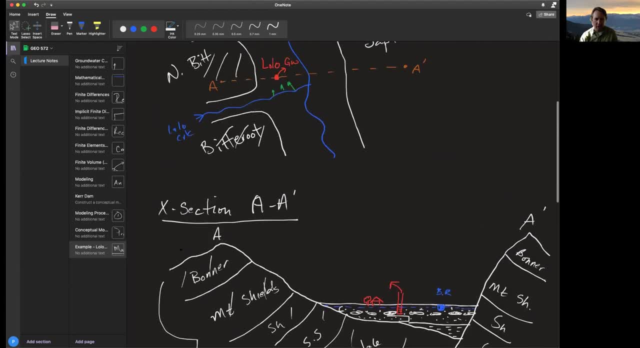 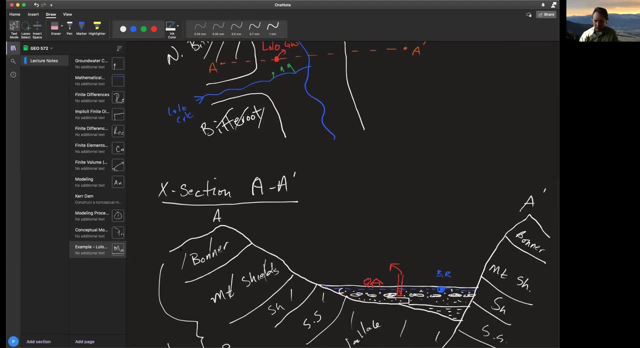 All right. so let's let's consider some of our important features here. All right, well, some of the important features. we've got this unconfined aquifer, All right, it's connected to the river and to Lower Creek. We've got these mountain block boundaries. 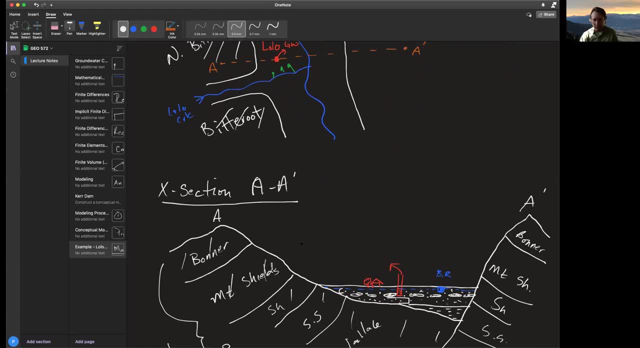 All right, so important features we might pull out here. So if we look at the top of the picture, there we've got a small amount of water, So that's the energy source, So the amount of water there. we're going to pull that out right here. 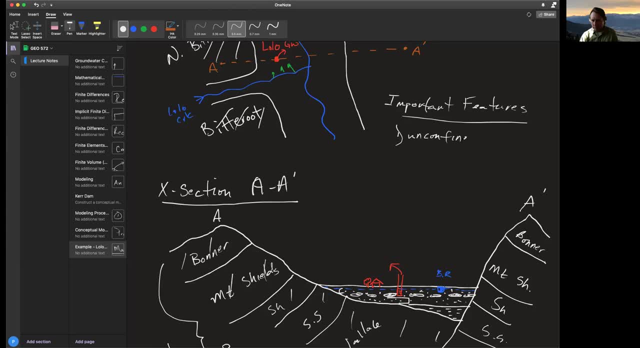 So let's find out if we can get a little bit more of a more of a statement of what we're trying to do here, So we can see that we have water on the ground surface And if we pull down the surface with the lens, 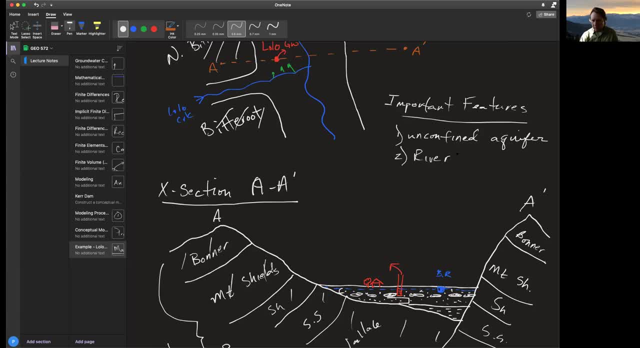 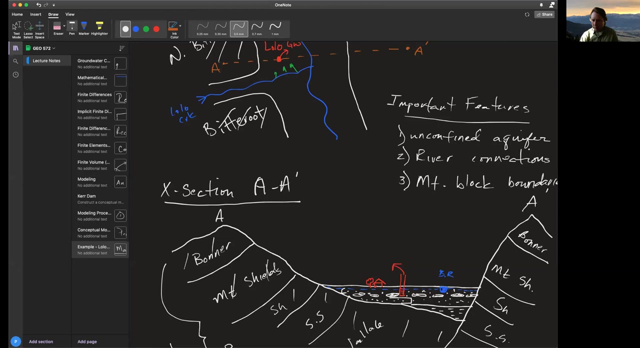 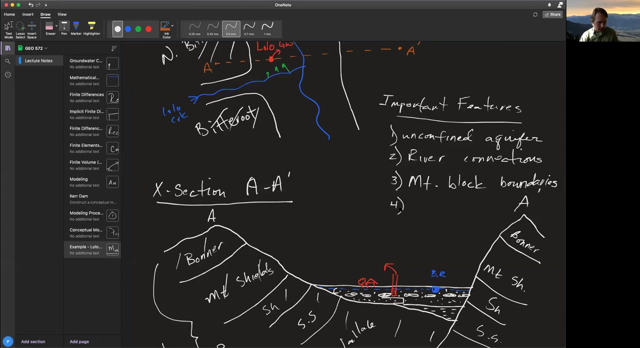 we're going to see a little bit more water on the ground surface In that unconfined aquifer. we have these mountain block boundaries. Beneath the sands and gravels we've got Eocene slash, Miocene Fine-grained sediments. 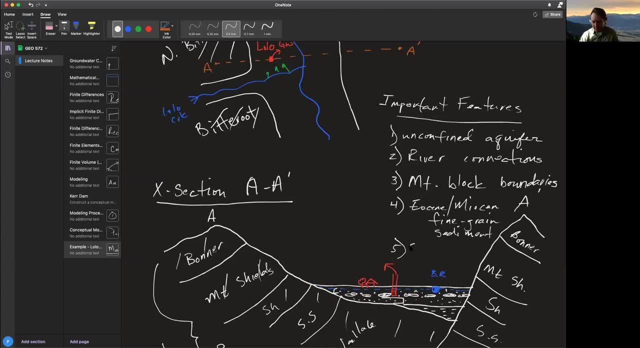 And then we've got this semi-confined. All right, Here's our sands and gravels. So these are the key features that we're going to have to consider when we develop our conceptual model. All right, So let's recall our ingredients. 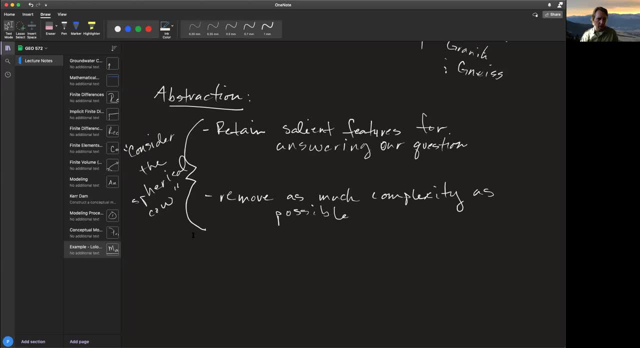 So the first was the governing equation of the important partial – the important physical processes and – which give us – well, we have an unconfined aquifer, So – 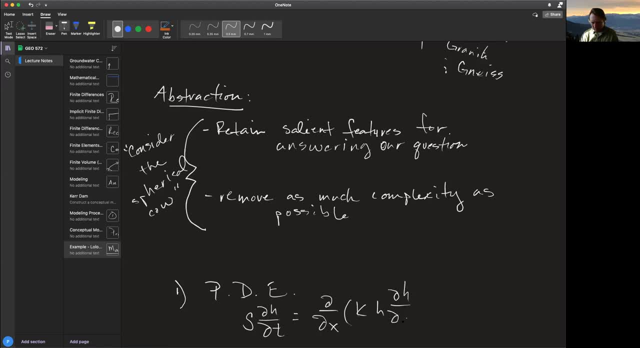 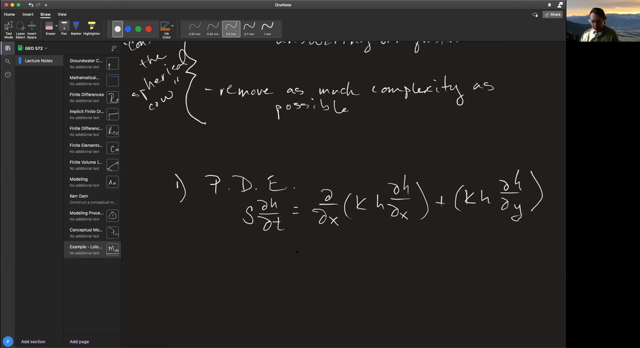 All right, Where this equation here is the unconfined aquifer equation, All right, and it has this extra head term in the spatial derivative. One question we're going to ask ourselves is: could we get away? this unconfined algorithm equation is much harder to deal with. we'll talk about how we deal with it in. 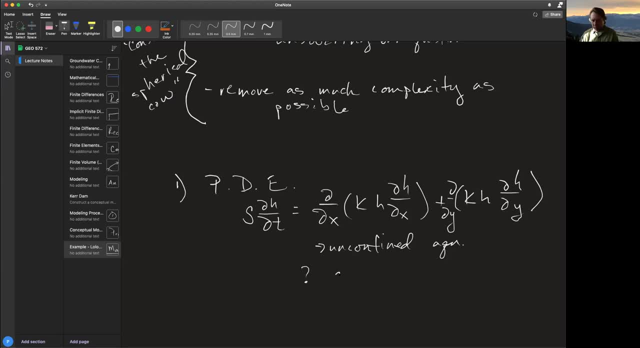 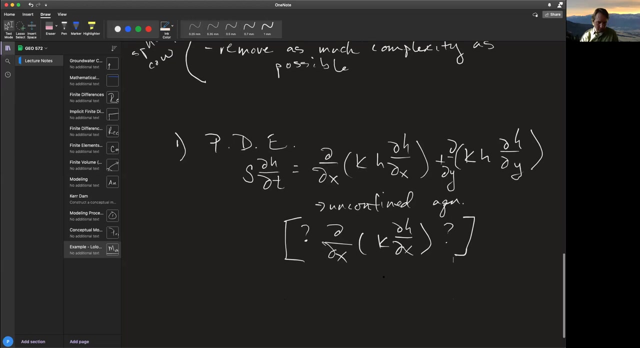 more modeling later, but could we get away with the standard confined algorithm equation? So one simplification that we're not going to make right now but we're going to keep in the back of our mind is: could we get away with simplifying to a confined algorithm equation? 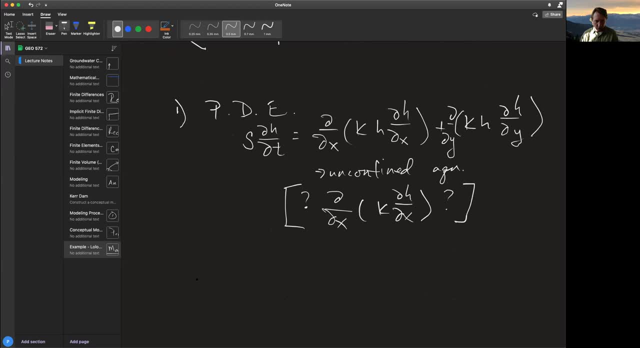 Okay, so the next thing is that is the domain, and this is one of the hardest things. so we need our domain of interest- And this is a really important and really hard move when we start to make our model- and that is: how do we isolate, how do we isolate the chunk of the world that we're interested in from the rest of the world? 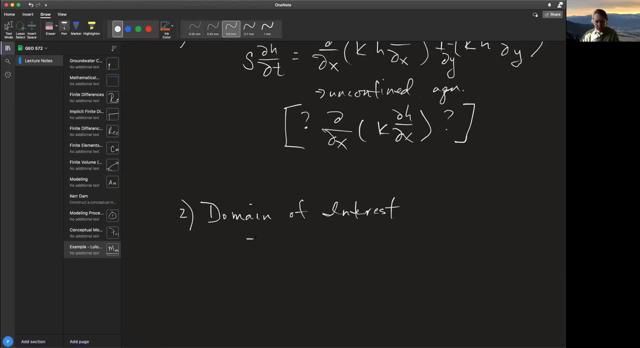 And there's some rules that we're going to try and use. So we want to use the minimum, Alright, we want the smallest domain we can possibly get away with. all right. we want the least number of dimensions possible- right, we can get away with a 2d model. we want it as a 2d model. we can get away with a 1d model. 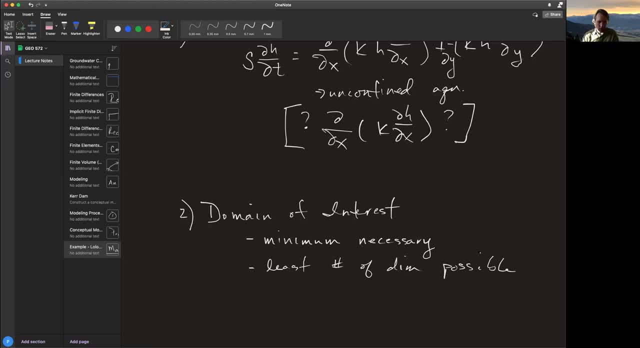 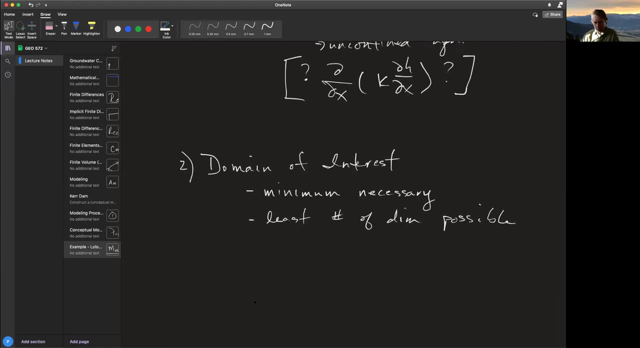 one thing that we're always going to do to help us reduce. so, for both of these, one thing, for these one thing to help us accomplish this is: look for lines of symmetry. all right, and what that means is if I were to draw a line, and, and my domain, 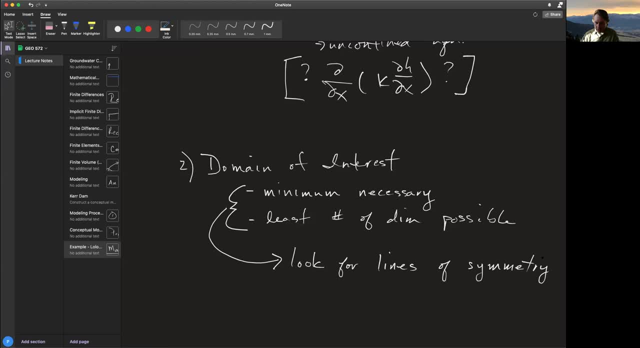 looks the same on either side of that line. well, that's a ends up being a place where I can just stop the model and get rid of a dimension or get rid of a chunk of the model. so symmetry is your friend. we're always going to look rely the same. 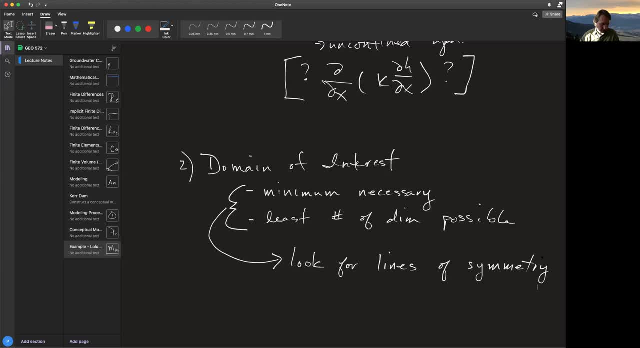 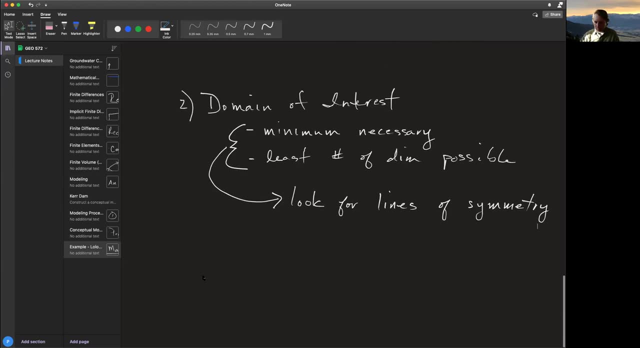 creature. we so some boundaries and some obvious places to draw boundaries, let's recall, first of all, so, let's, let's say that one of our key moves here is to come up with boundaries and we're trying to define all obvious places to draw boundaries. well, let's, let's recall totes sort of. 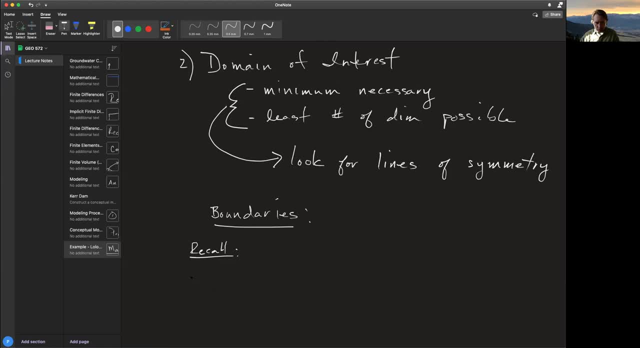 two-dimensional groundwater model where we had this sloping, undulating water table and, if you remember this, from intro to groundwater, you can solve for the groundwater flow in this. in this kind of situation- and when you do, often you raise the wrong one, and when you do, 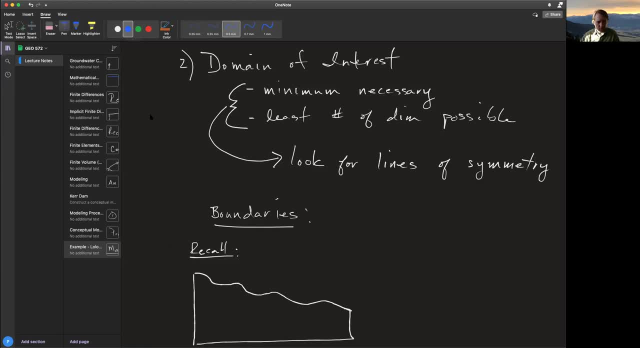 you can get a different kind of flow path and different color when you do get these short flow paths that flow to adjacent streams and get longer flow paths that flow to distant streams and, depending on our system, we can use these flow paths and this configuration to think about something natural. 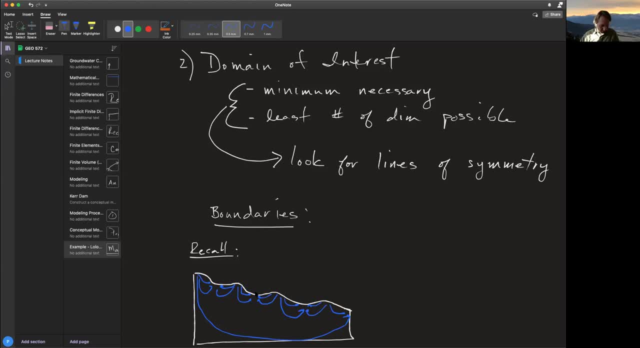 okay. so, first of all, there's watershed divides at major streams, alright, so water is not crossing underneath major streams. so some obvious, obvious places. streams are often divides- not always- but strings can be good places. any kind of vertical structure might be an obvious place to stop changes in hydraulic conductivity, which 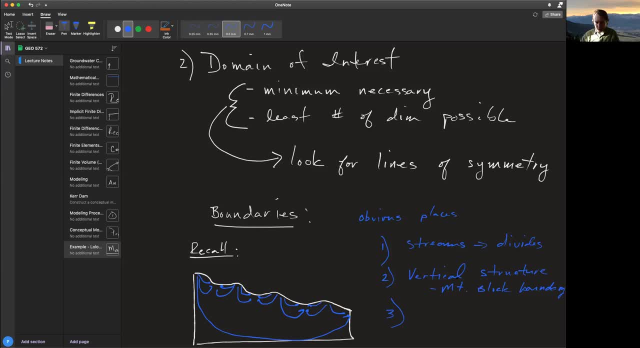 is really what a vertical structure might be, just a vertical one. so anything where the hydraulic conductivity changes and specifically where it gets really low and where K is low, that might be a natural place to have a no flow boundary. so we have a couple different things to think about here. so first of all, there's a watershed divide on the ridge. 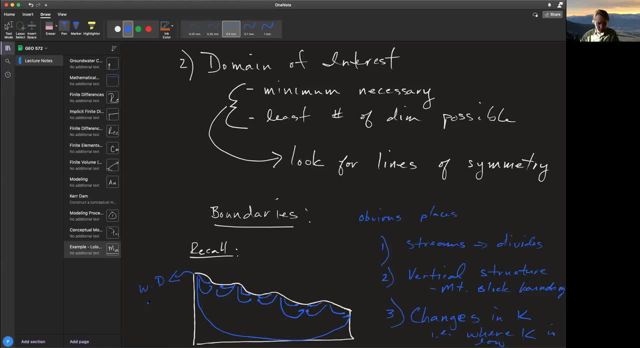 on the regional ridge. there's a watershed divide. on the regional screen it's a ridges and streams and natural places. if we're not interested in deep flow, then local. if we're only interested in the flow into the shallow zones, then a local ridge and a local stream might be a natural place. so you can have a boundary. 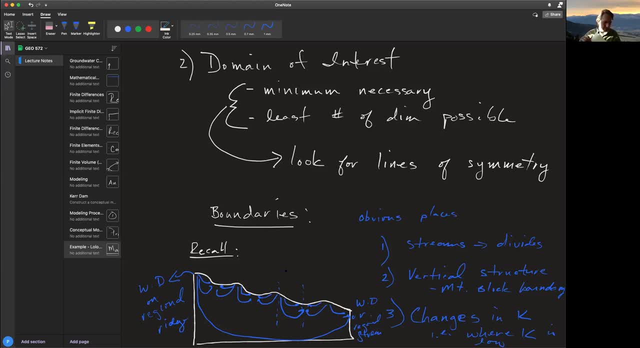 okay, so those are. it's really there's no right or wrong way to draw the boundaries, but these are natural places to draw: Vertical structures, changes in hydraulic dynamics, streams and ridges. These are natural places that we might say, hey, there's no vertical flow or 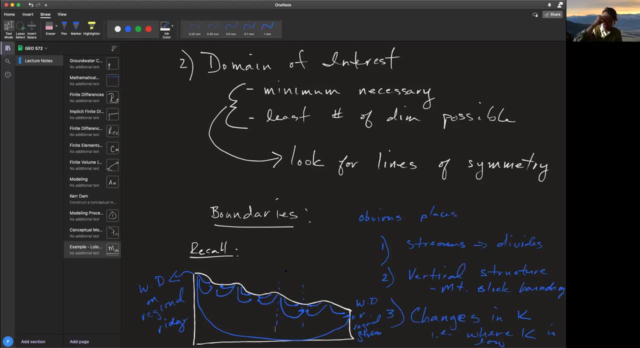 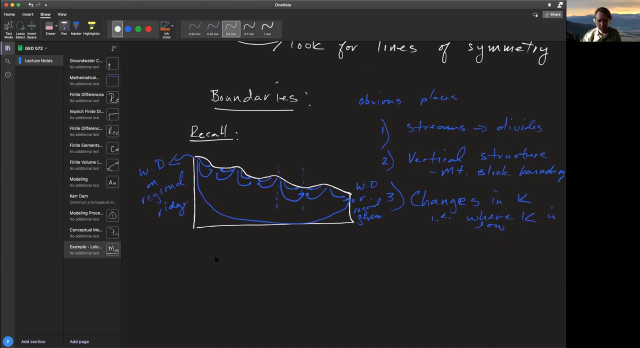 there's no horizontal flow across these zones that we care about, so we're going to call these no flow boundaries. Okay, so that's how we define boundaries. The next step is: well, we've got to think about what kind of boundary and the 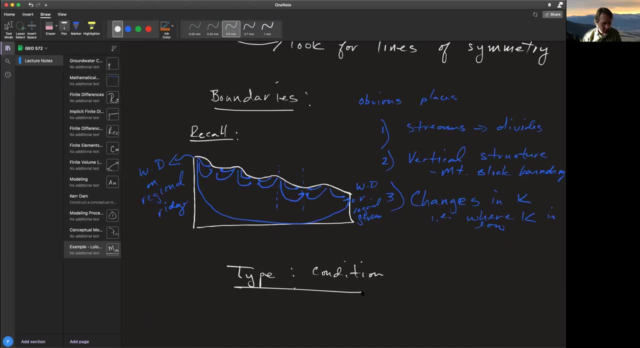 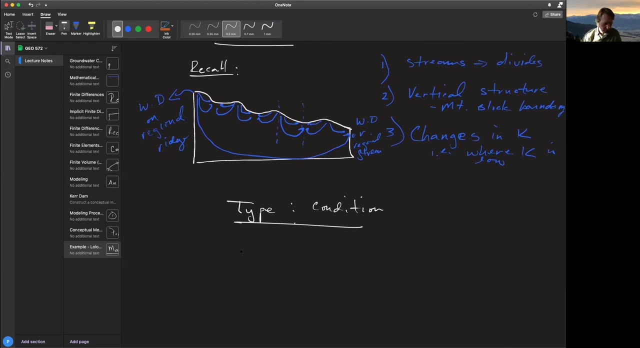 condition, All right. so we have a few different general types, but one is first. one is a known head, all right. Well, a place where we might know the head is in a stream, all right. So streams are a great. 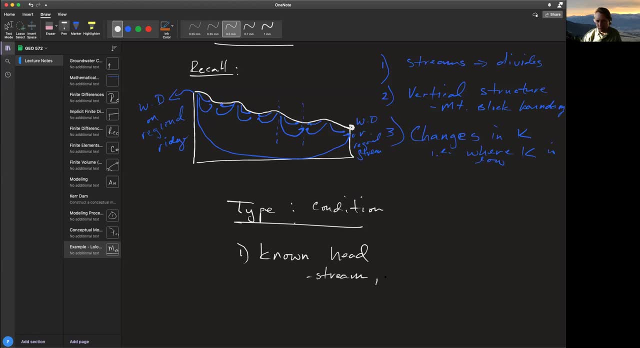 place Stream, a lake, ocean, All right. these are places where we know the hydraulic head at the sign or in the model or in the domain. We know what the elevation of the stream is. That's easy. 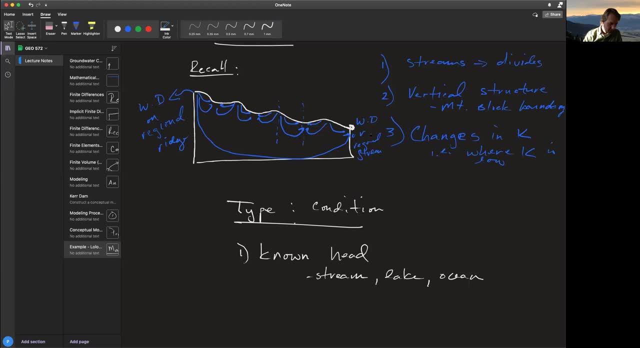 for us to measure. We might also know the head in a well or a series of wells. all right, So these are places where we can set boundaries. Um, so then the other, the second type, is a known flux. all right, Remember, this was our. this is the first, one is our. 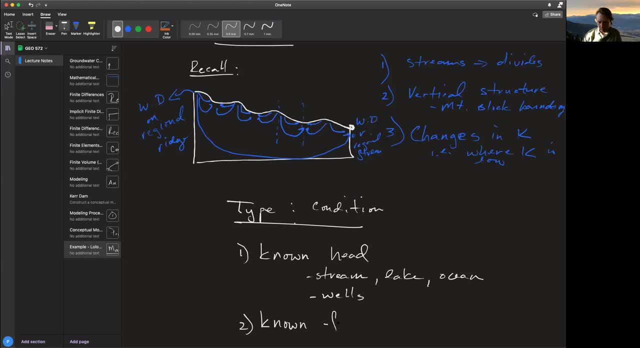 Boundary. This is our plug-in Boundary. all right, so now we need to get to our, our impression of the road. So if you can do this in just a couple of ways, 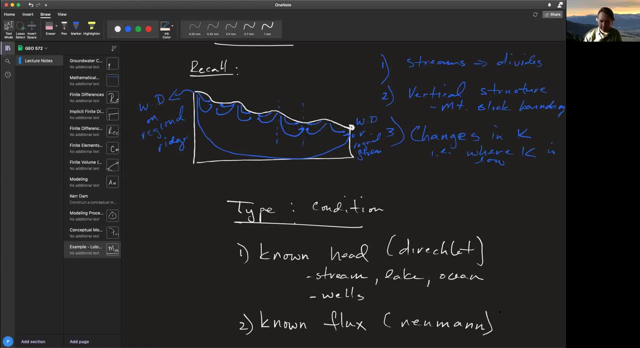 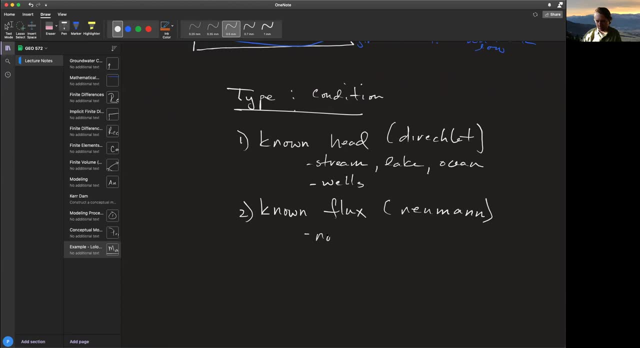 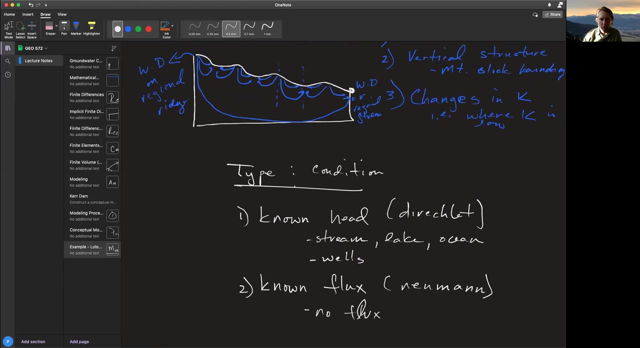 known flux. well, first of all, no flux is a subset, so no flux. well, let's think about this. like: look at this regional bridge up here. there's no flow paths here that are crossing over that bridge. so this is a no flow in the X. 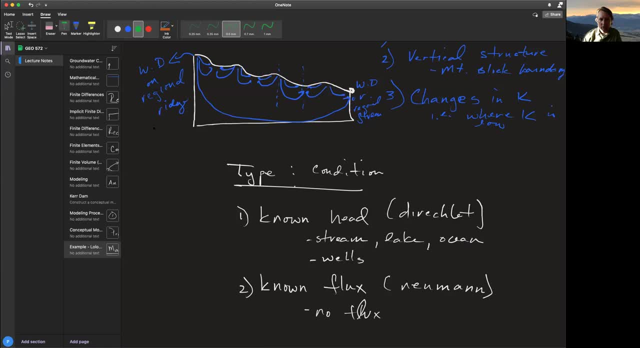 direction or in the horizontal direction. so this is a no flow in the X direction. similarly, if all these groundwater paths are coming up and discharging to the stream, there's another no flow. all right flow can occur along the boundary upwards. it is not crossing all right if. 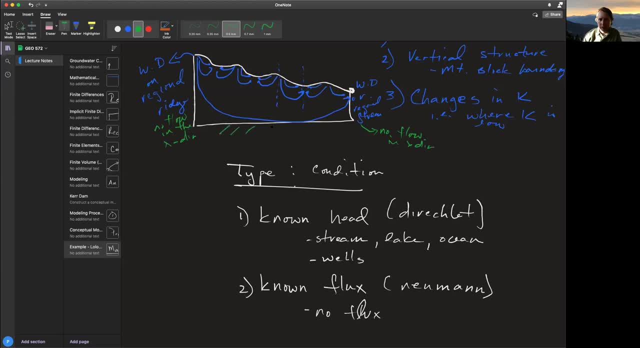 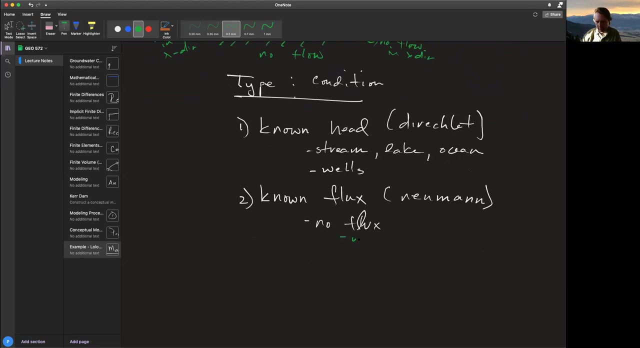 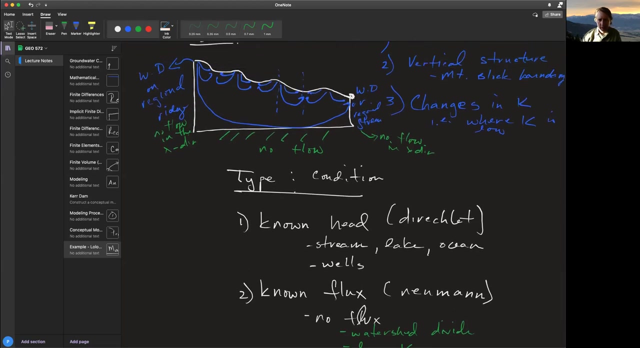 there's some low permeability layer down. it's preventing water, right. so no flows are watershed divided. now there's some tricks here. how do we know it's the regional zone? how do we know there's no lateral flow? we don't At some level, like in the US. the continental divide is the regional, the largest regional. 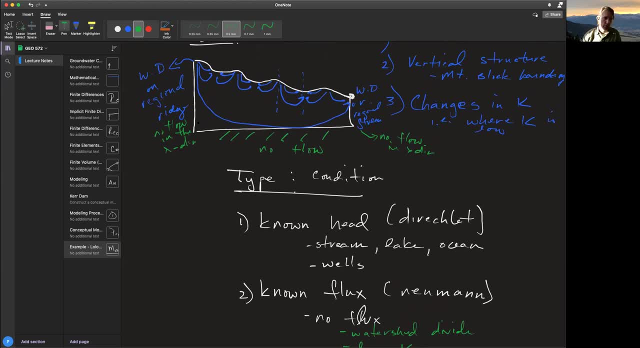 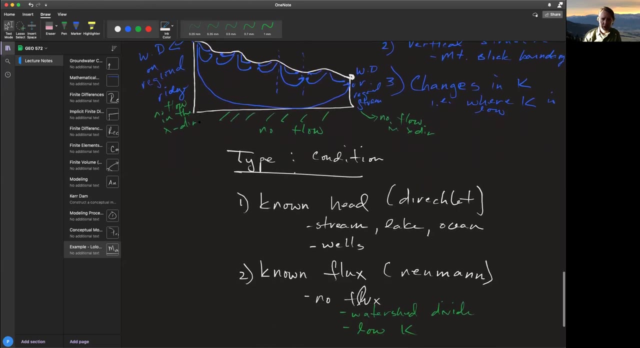 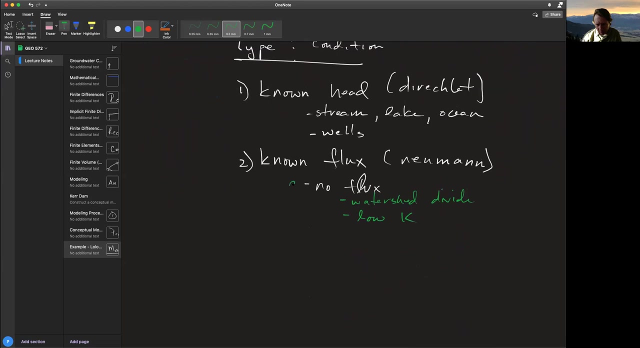 divide, So there may always be some degree of regional flow that we're not accounting for. However, it's very, very small in the hydraulic conductivity structure, means that the flows are kind of very shallow. Okay, So no flow is one subset, so that would be A And then B are just any other known fluxes. 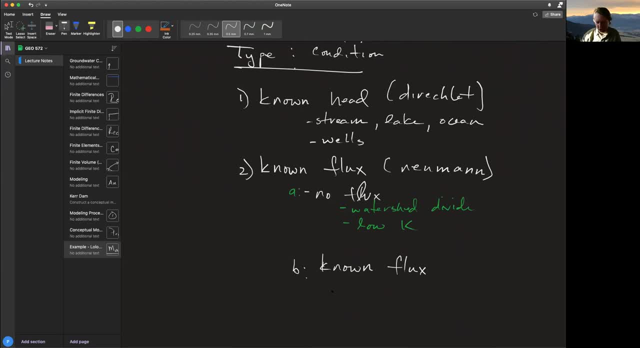 So, for example, irrigation, Okay, Okay Okay. Injection wells, We might be able to approximate the recharge rate Any place we can sort of Side. But hey, across this boundary we might know be able to estimate flux. 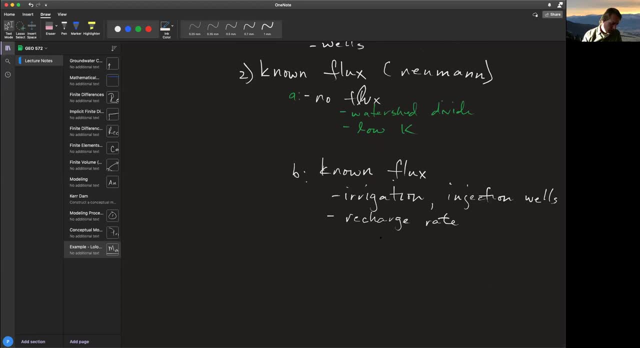 And then there's this third type. it's a mixed, All right And, as an example, Okay. So, for example, one of those might be a spring. A spring, we only have discharge when the groundwater head gets above a certain value. 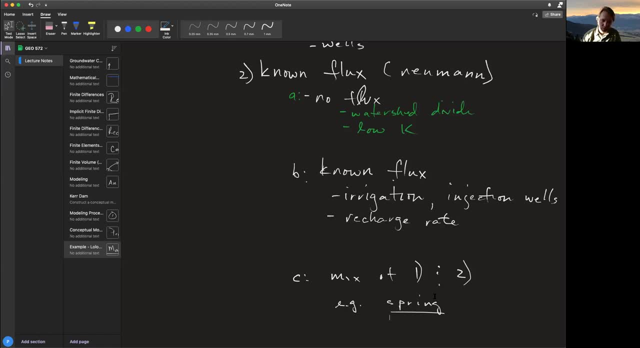 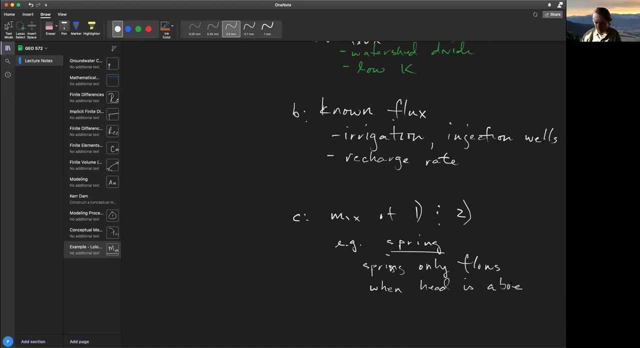 but then, once it achieves that value, it will flow out at a certain rate right. So a spring has a mixture of the head. So a spring has a mixture of the head, of head and hands Screen on the clothes. How does God glance at this? 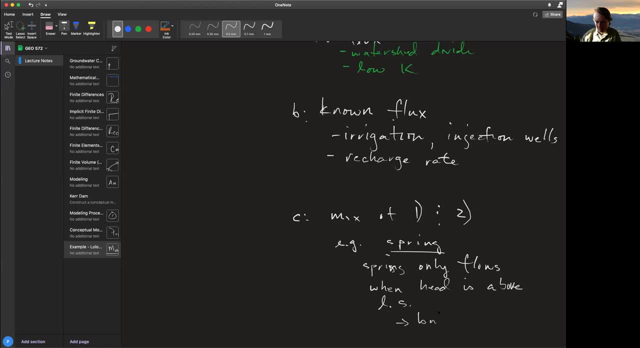 But then it flows out of your head. Come on, So it's a mixture of some have to combine some knowledge of the value of the head and the joints. Okay, so when we, any time, we derive our boundary, we're going to think about what kind. 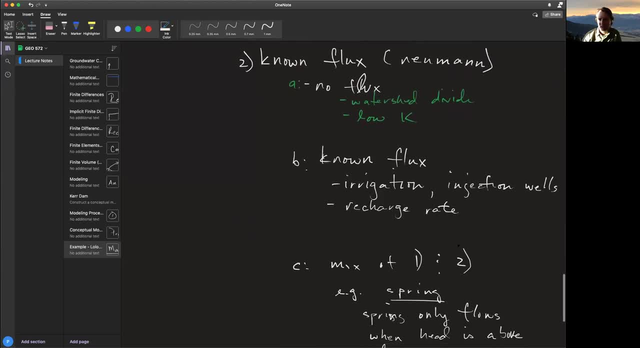 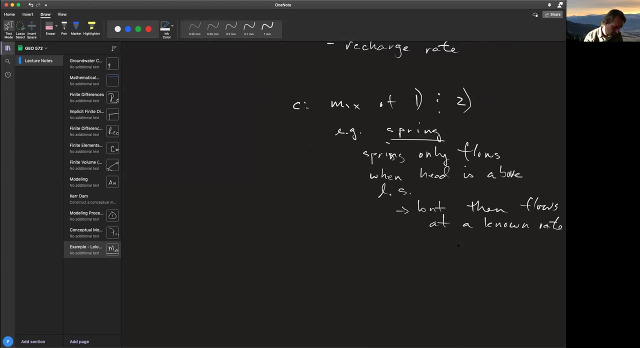 Do I know the head Or do I know the joints? I have to define one of those on all boundaries. I have to have some boundary Initial conditions. All right, and this: how would the system look when we started to do anything? 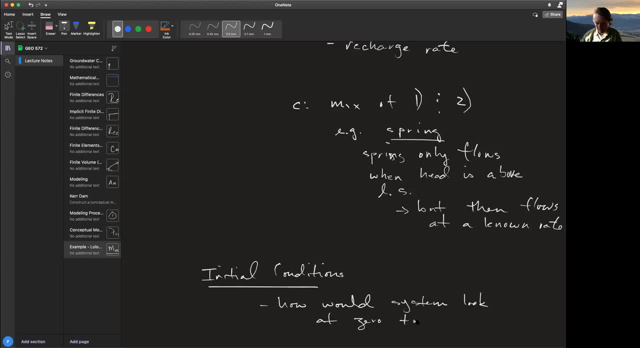 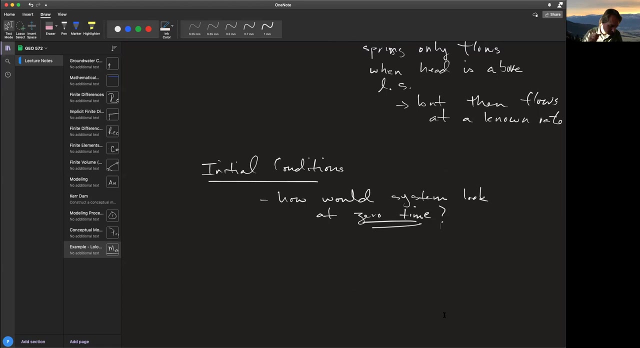 All right, and I just want you to think about it. This is really hard. What would the system look like at zero time? What is zero time? It's not real, So we have to come up with some approximation. that's a reasonable starting place. 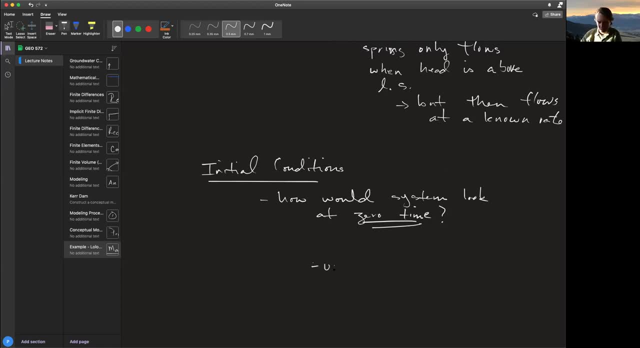 So some examples might be the head's uniform. I just can't. Let's say This is like: well, the river, my groundwater, is perfect, All right. one way we I often get initial conditions is to have a boundary. 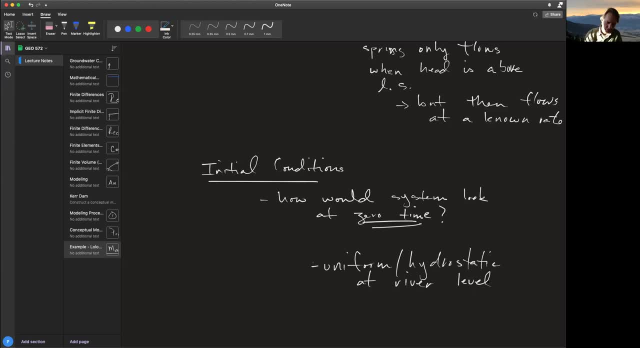 So I have something that's sort of nonsense, like: okay, the river and groundwater are in perfect condition, It doesn't exist. But then I will then add, use that as a starting deviation, add precip or whatever, and run that for a really long time. 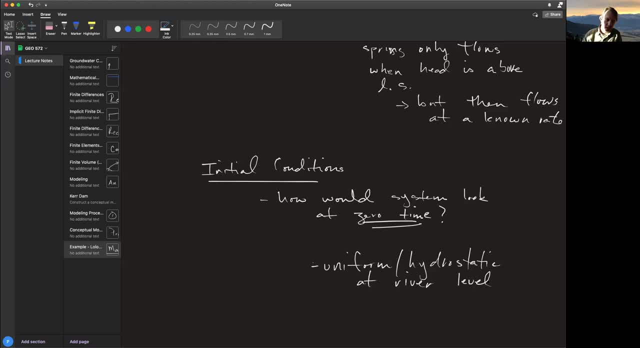 and get that sort of long time as the steady, as the initial conditions for another model in which we start stressing models and say what's the boundary, Okay, And that is called spin-up. So one way is to spin up is to get our initial conditions from the spin-up. 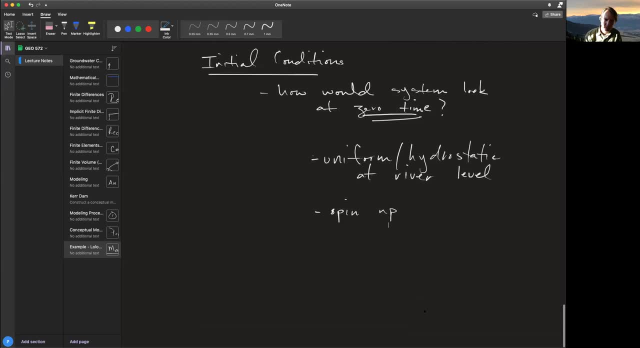 So we run a model for a long time and then we use that as our initial conditions for the next step in the model. All right, so we've got the boundaries, we've got the model domain, and then we've got the boundary conditions. 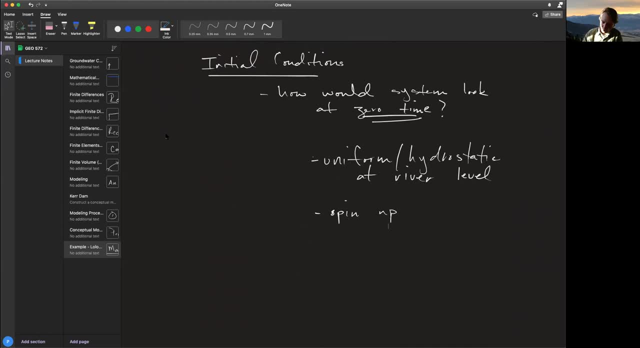 Initial conditions, And then we have to think about parameterization, right? So what are? what does the subsurface look like? Okay, So we need to consider a subsurface structure, And how does that lead us to be able to define? 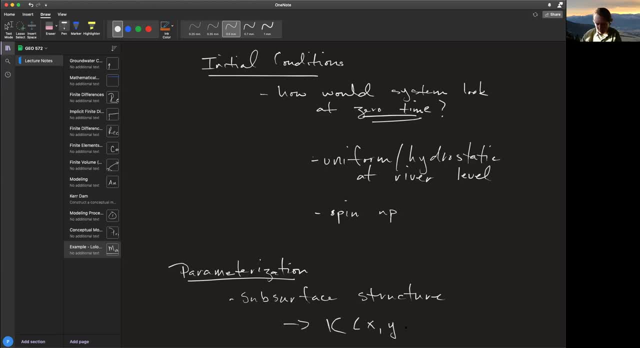 say, hydraulic conductivity as an optional space At each one, at each location, I'm gonna have to define the hydraulic conductivity, All right? so when we're so, this is our job. We've gotta come up with all these things. 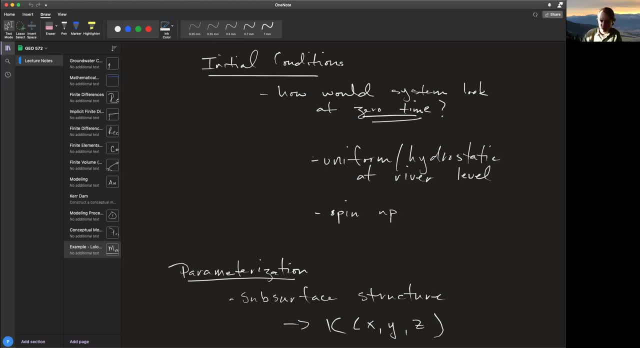 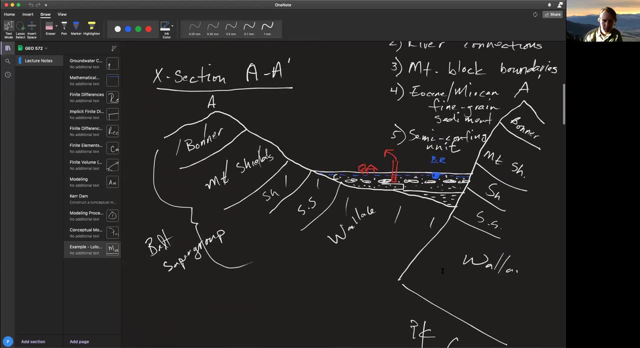 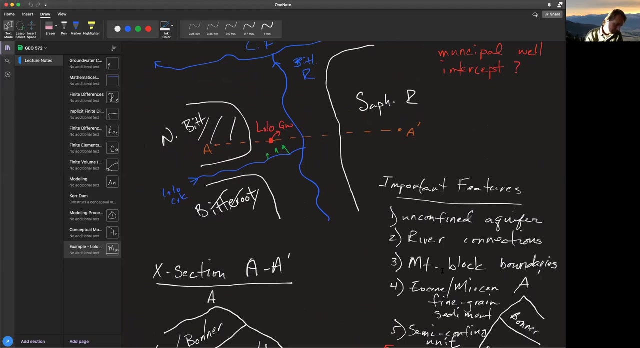 And when we do it, we're gonna wanna remember all of our assumptions so that we are honest about our uncertainty. All right, so let's go back to our example And let's look at- let's look at- what might be some reasonable boundaries. 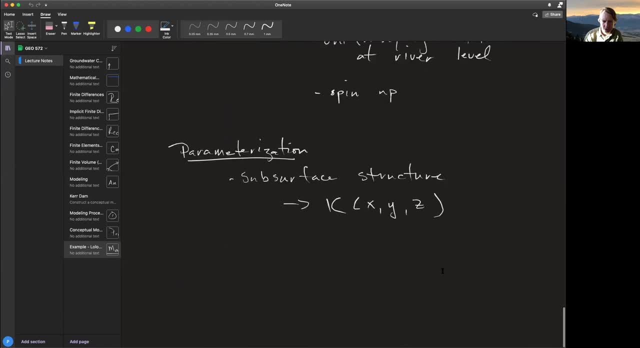 All right. so I'm gonna go back and I'm gonna redraw. So back to our example. I wanna redraw some of these, or draw some boundaries, using these principles and think about: well, what am I gonna do? So here's the first thing I'm gonna do. 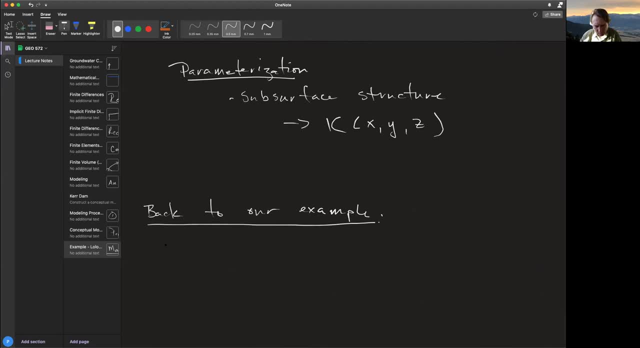 So let's start off with cross-section, Because this, in many respects, is the easiest. So, if you recall, we had sort of this mountain front coming down a mountain block And we had a mountain surface and we had a river. 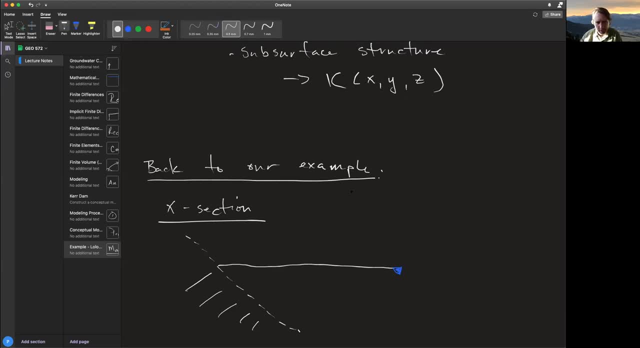 And we had, And then we had this low permeability layer of renover. All right, so there's some natural boundaries that we might cross. Well, first of all, this: Oftentimes we think of the mountain block, as these mountains are low in permeability and sediments. 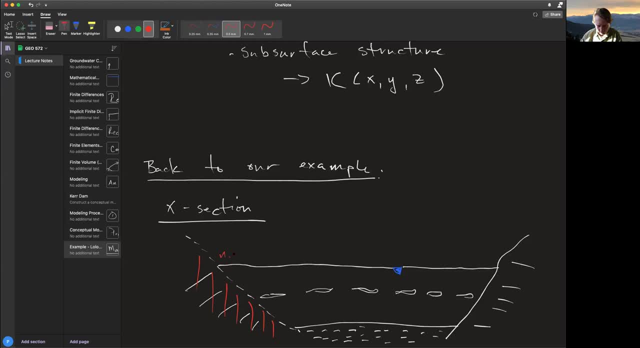 So we might say, hey, here's a natural boundary for the flow of conductivity, And so we might say, OK, there's one boundary, And it's a middle flow. And then we might say, well, this river's a pretty big river, a regional river. 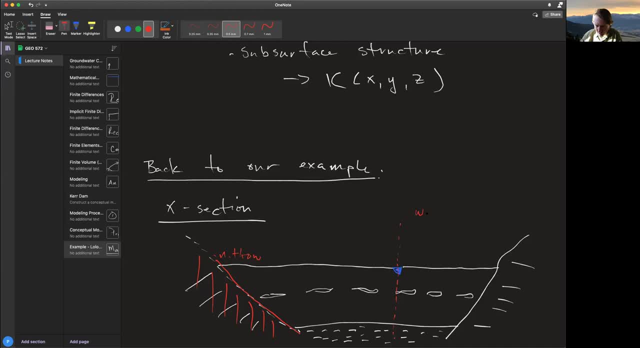 But it's not going to be a watershed without a crossing. This is no flow in this direction. All right, OK, now let's think about, well, this guy's low permeability. So we might say, OK, no flow here. 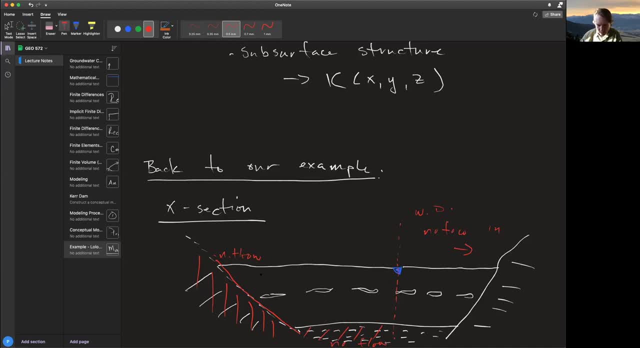 Right, No flow from the renova. Now we have one more boundary to take care of, All right, and that's this top one, And we might apply a recharge flux here. All right, that's some amount of water that falls on this land. 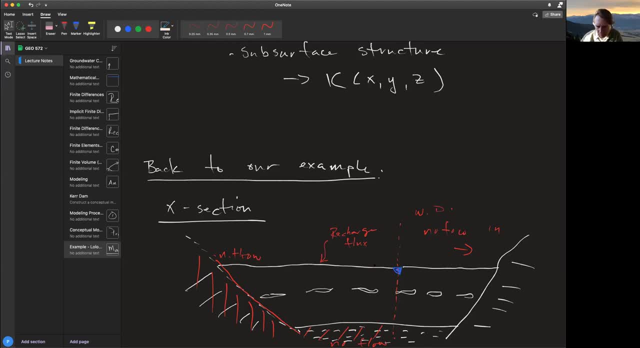 And it's temperature and soil OK. so we've simplified our model domain And again that's just a little bit of a in somewhat reasonable spots, All right, And so I've got no flow right here. But on this boundary, 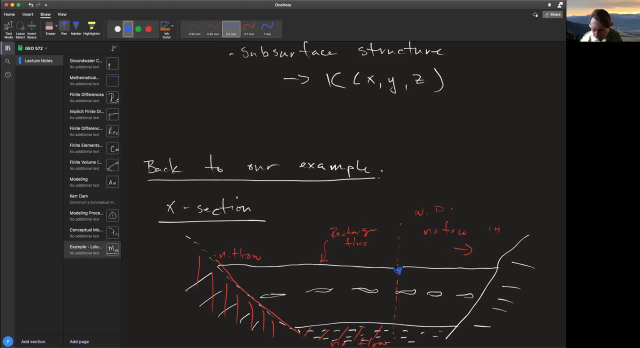 where the stream is boundary condition, where it's specified like equal to the temperature, All right. So we charge across the fan surface draining to or infiltrating from the river, and it's no flow on the boundaries of the top wall down into the nova and the middle of the river. 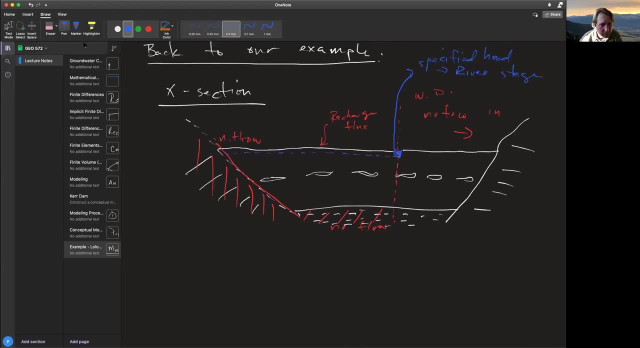 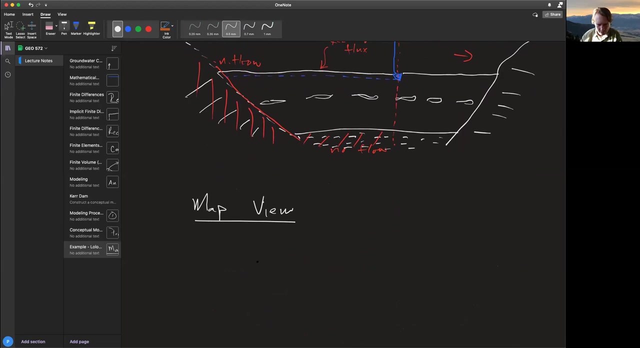 Now let's look in the map view. Right in the map view, remember we had sort of a park forks coming here, a bit of a roof coming here, a little creek coming here. So I'm looking for a line where there might be a signature here and while it's not perfect, 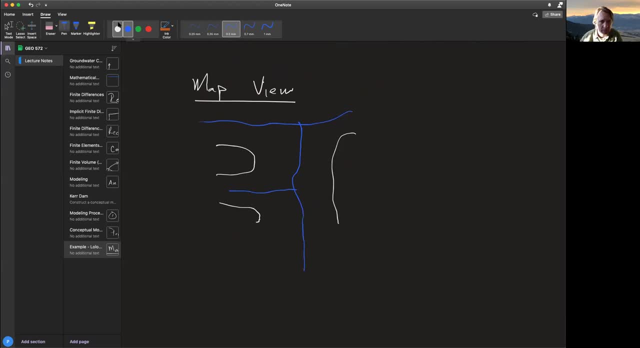 symmetry and you might get called on it. you're going to have to justify the area where I can see a natural boundary. It's not good symmetry. It's not really symmetry, but we might say, hey, there's a roll of creek here. 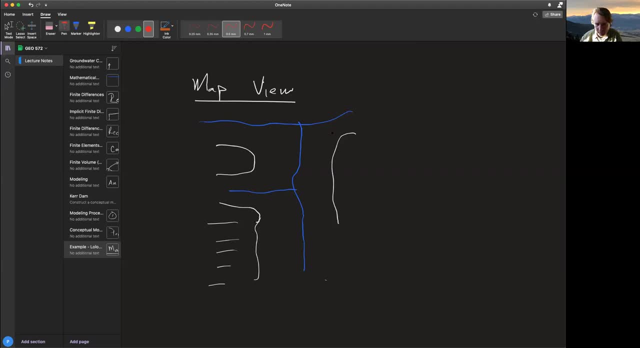 All right, now remember, we've already gotten rid of all this stuff here, so it's gone. The next question becomes: all right, everything on this side of the river is gone, and everything on this side of the mountain block is gone. 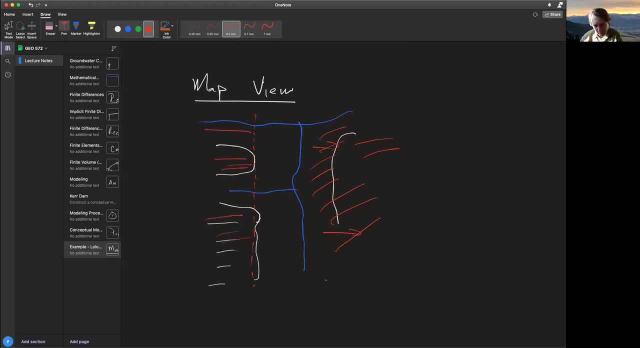 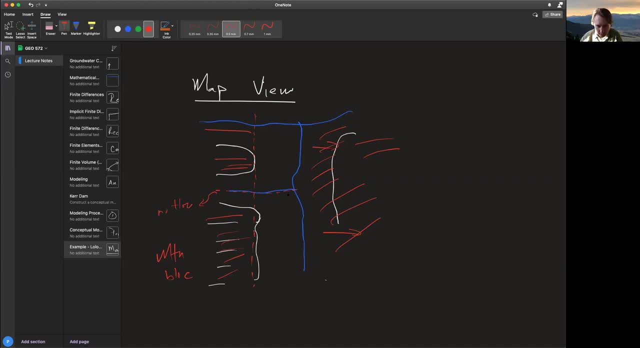 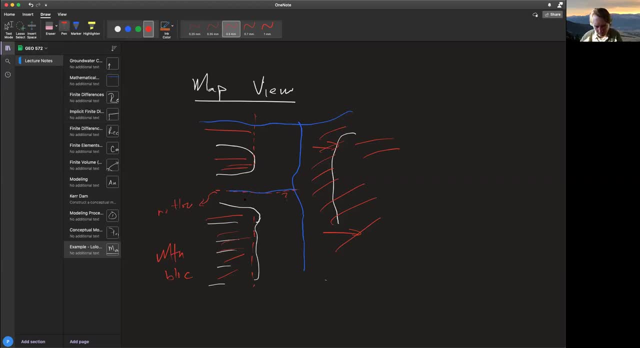 So we don't even have to make it. So it's just going to be a pretty little thing. All right, All right. So what we're going to do is we're going to go back to our log. So we have a little bit of a line here and we're going to cross out all of this. 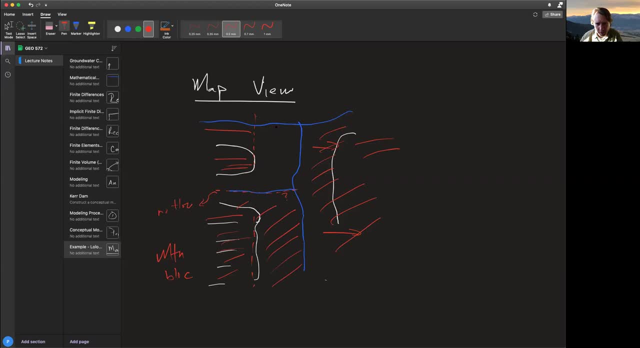 So that's a little bit of a line, And then we're going to cross out all of this. Now my model domain is here and I still don't have any boundaries here, and it's unclear how I would draw this boundary. One option is to say, oh well, how would I know? there's some wells up here and maybe. 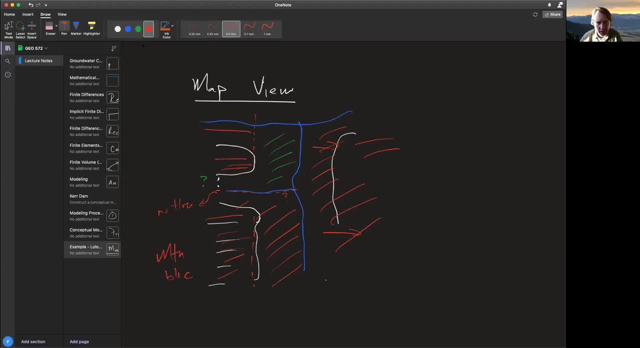 I can draw a constant head down here where there's a well zone, Maybe All right. One thing we can do here is the farther we move this boundary, the more we can draw a constant head down here, and the farther we move this boundary back up, the more we. 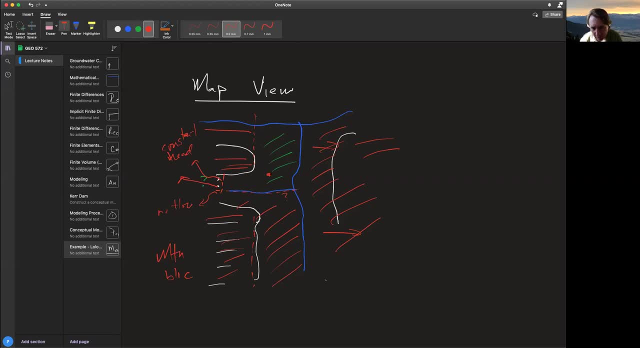 insulate our prediction of interest. Remember, what we're after is how much water from the well is going to this well. So if we move this boundary upstream, we insulate how much water is coming out of the stream to the well. All right, 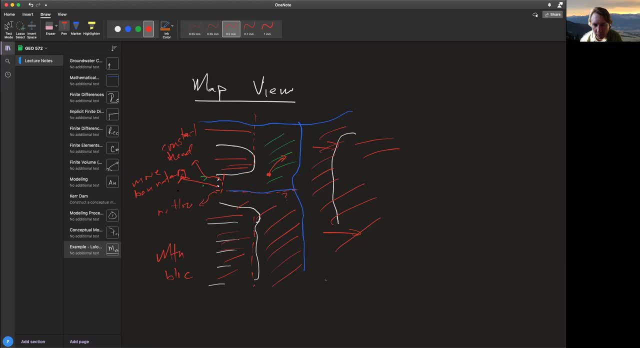 We'll just move our boundary away from it. So the farther we go Your boundary is away from the prediction of interest, the less influence it will have on your prediction. So if you don't know what your boundary is very well, then you've got to move them away. 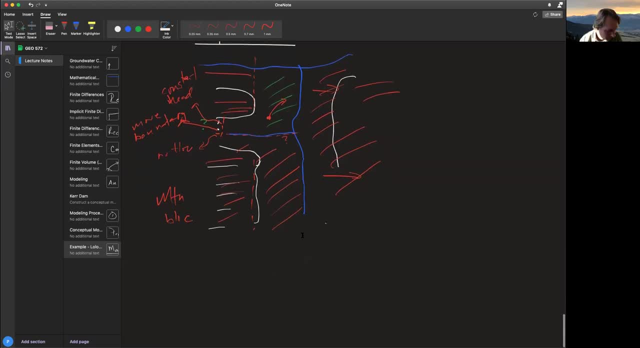 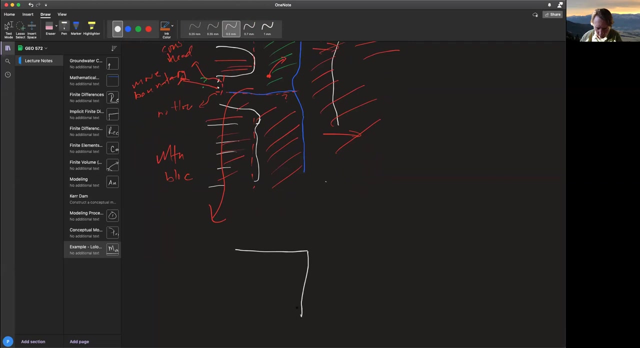 from your area. Okay. So I think, if I sort of extract this now, we've kind of got this kind of a model, It looks like a box. This would be river head. Okay, Okay, Okay, Okay, Okay Okay. 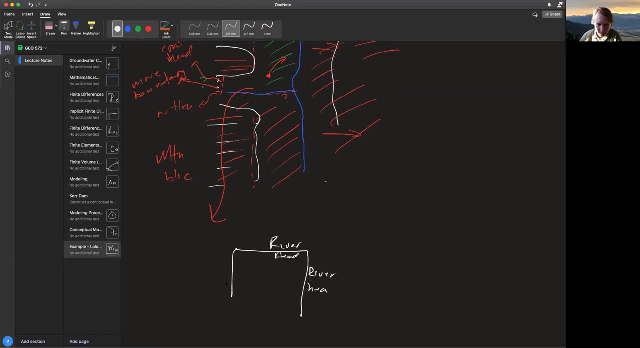 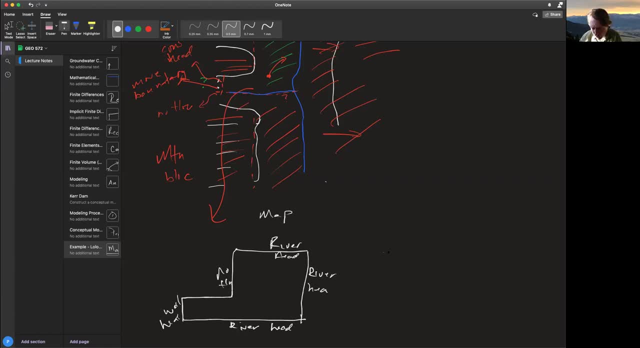 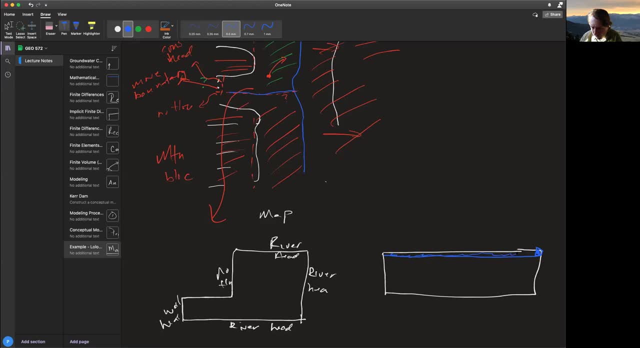 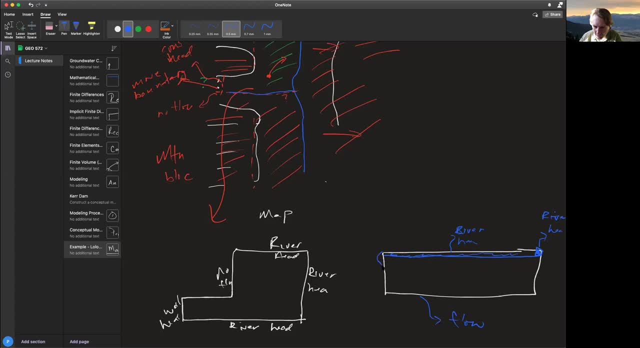 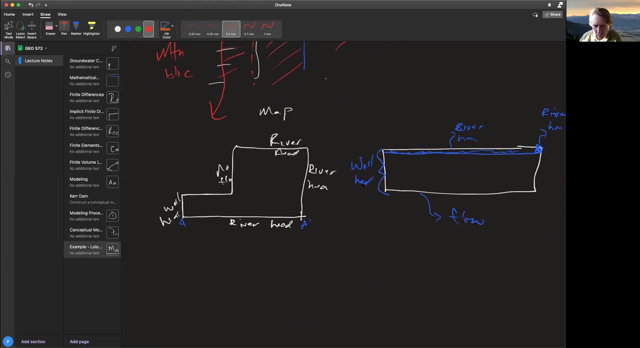 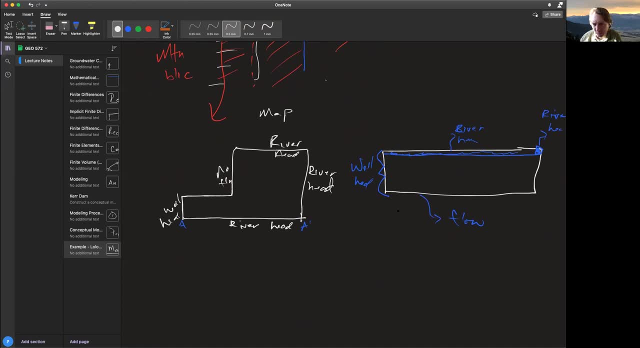 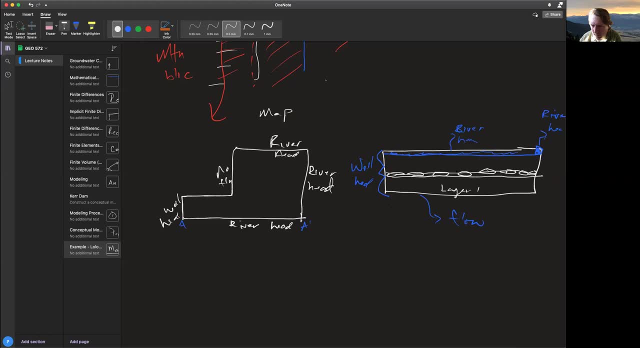 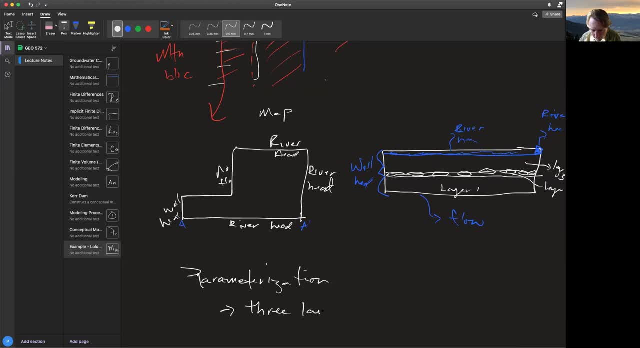 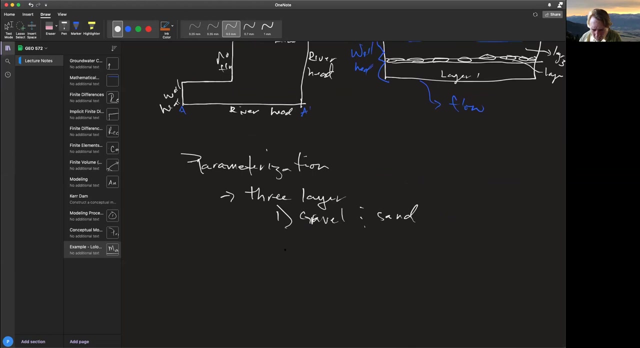 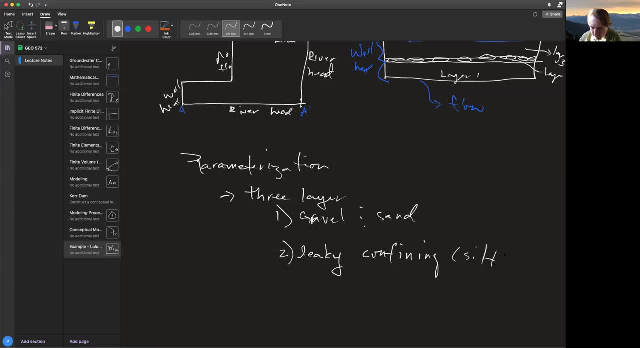 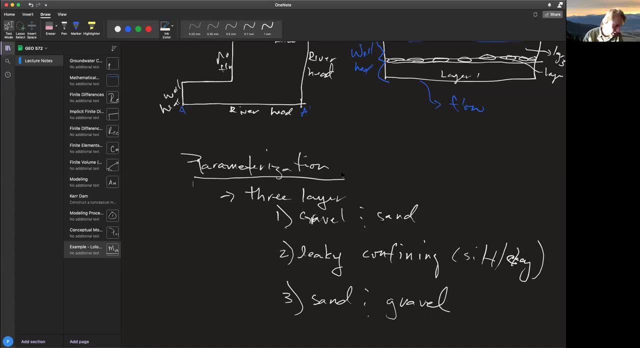 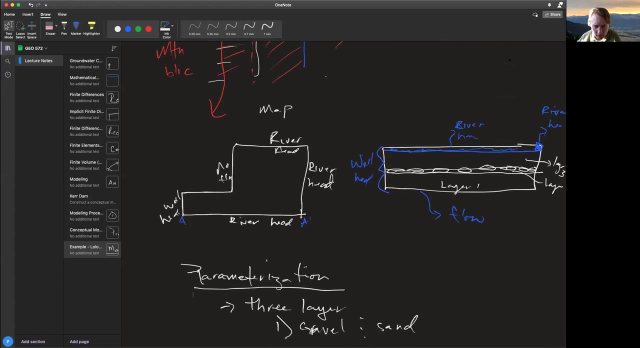 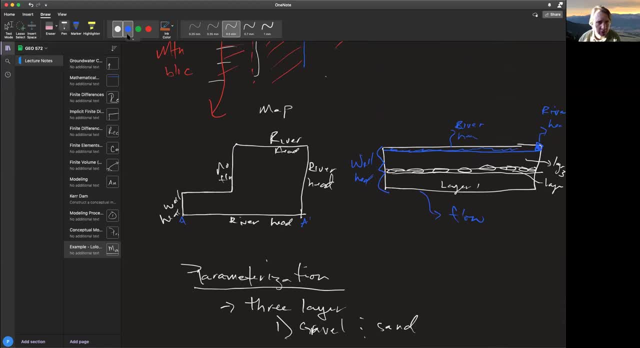 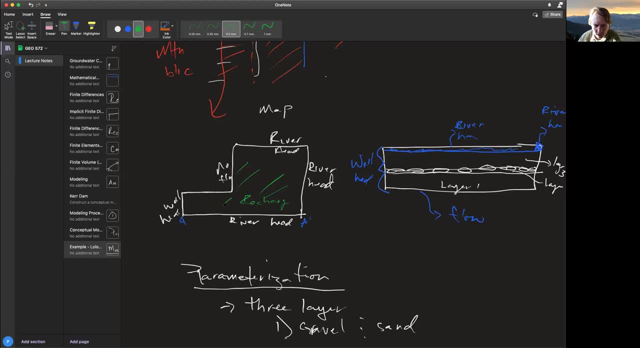 the alluvial aquifer And then across the entire surface. I'm going to have a constant edge. I said: well, you know, the things I'm most interested in here really is just this stretch out of the river and it feeds my well, so I don't even consider moving it to. 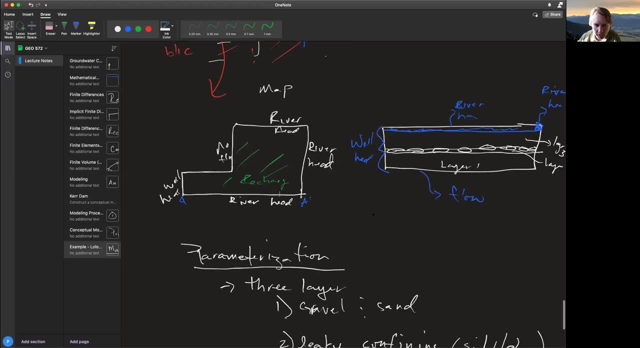 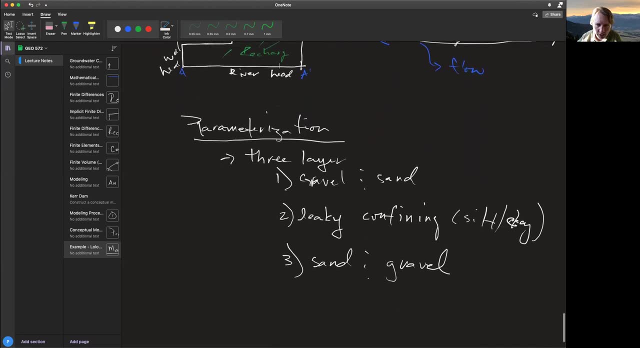 the most active layers in the alluvial aquifer. So I said, okay, there's three layers you know. Now, I know about. you know well, how would I you know when I, when it comes to actually 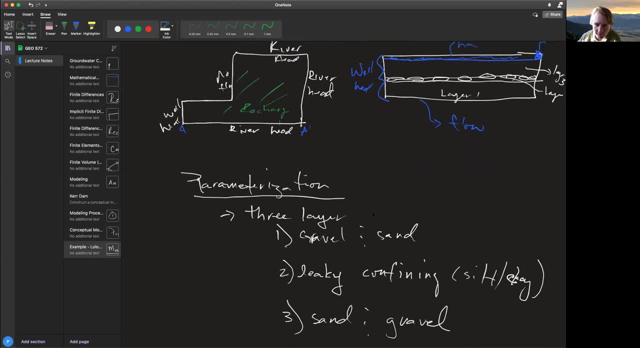 building a model. I better think about how I'm actually going to take the values into account. I've got to figure out how I'm going to calculate the future. If I'm going to apply this as a boundary condition, I better be able to, you know. 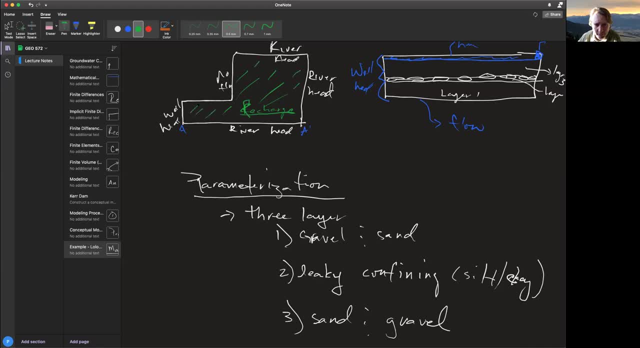 figure out what it is Your top tip. it's going to be hard, Okay, So we've ended up with this conceptual model. A few things about this conceptual model. It's not right. It's not perfect for sure. There's lots of potential problems. 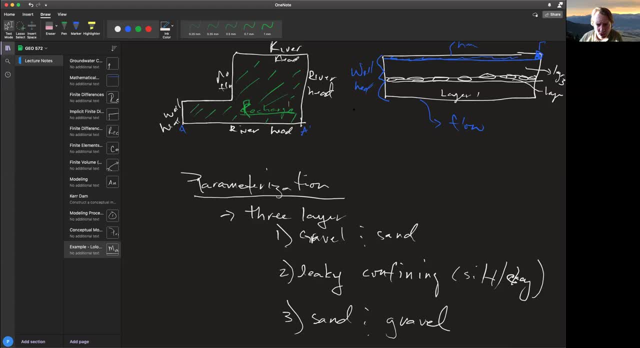 We've assumed that the river's. you know it's going to, you know it's going to be great for downriver management, but you know it's going to be a lot more local than it is, for you know river management. 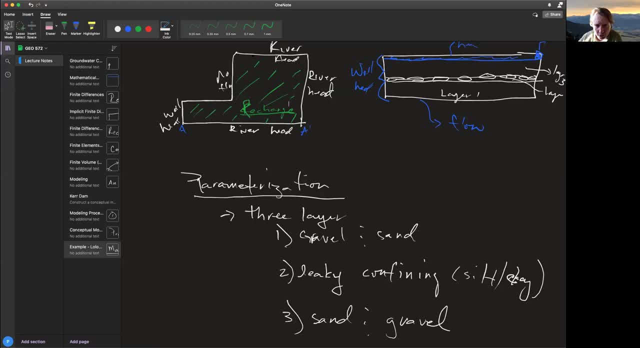 And we've assumed that you know a lot of the rivers don't allow any sort of regional flow across them. That's probably fine for bitterroot and we've assumed the mountain blocks are more flow. A lot of what I'm working on in my research is deciding whether that's true or not. 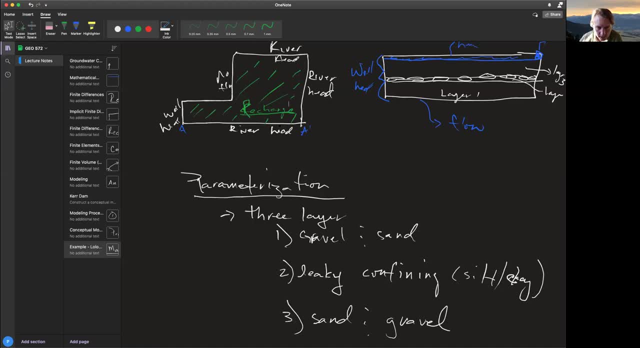 I don't know what it is, I have no idea, I don't know, I wouldn't be able to confidence. So I think you know we're using now. we're using the stuff that we've already learned about the lake. 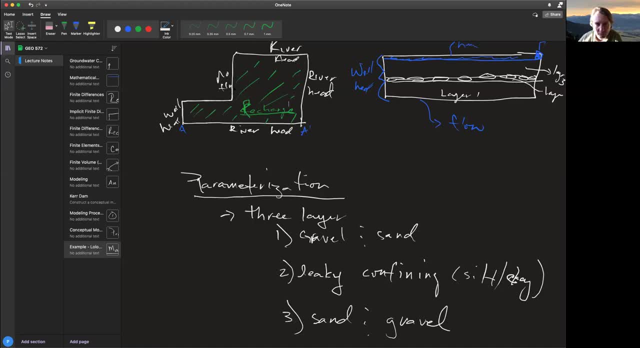 So that's another thing We're going to try to say: you know, you know it's a threat in this, in this, in this case, It's going to be great, or just deciding whether that's true or not. 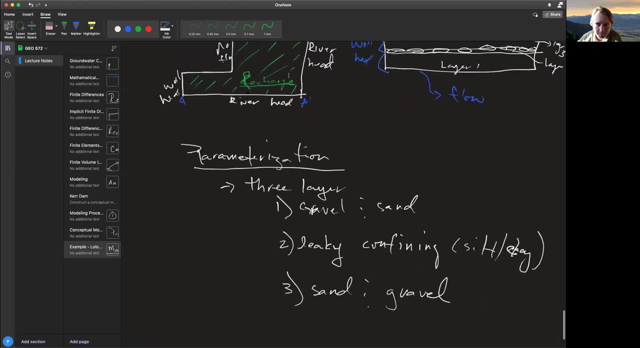 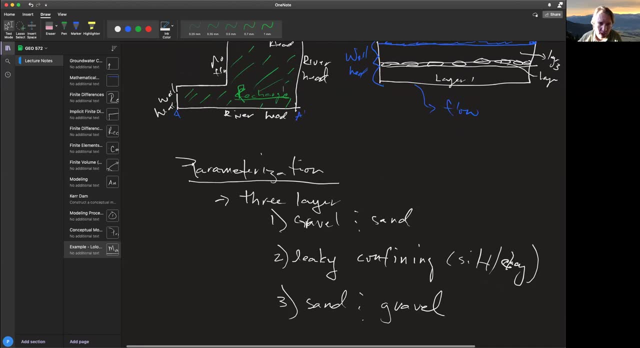 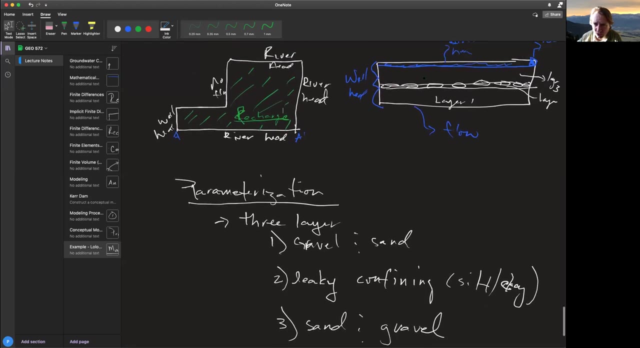 I don't think it is. I have no idea really what to do with this boundary condition of low-level, but we're gonna approximate it and move it far away from our. We've also assumed three layers, And maybe that's true and maybe it's not. 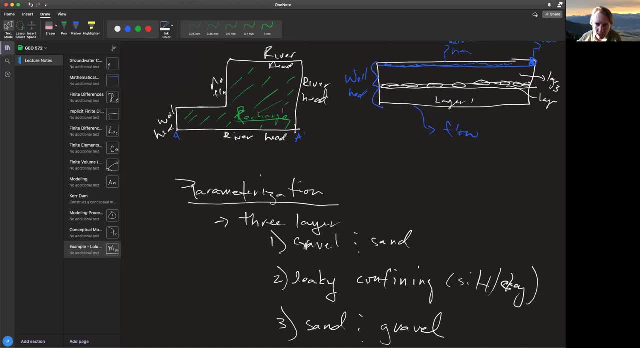 We're sort of approximating these lenses of silt and sand as a single layer, Or it may not be okay, right? So bottom line is: it's not perfect. It's suitable to address our question. It's suitable to address our question. 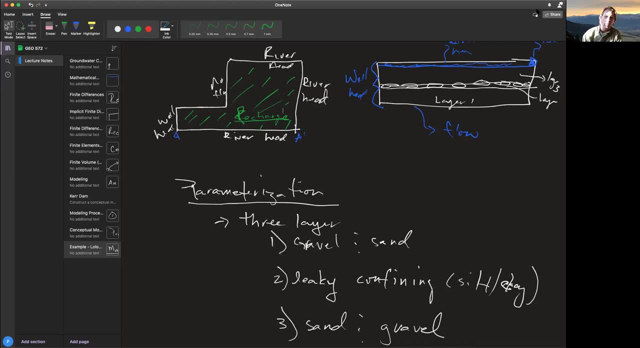 We can ask: well, how much water can low-level trees need? Or how much water can low-level trees need to come to our well? It is a reasonable model. It's designed to focus in on that, But when we try to answer that question, 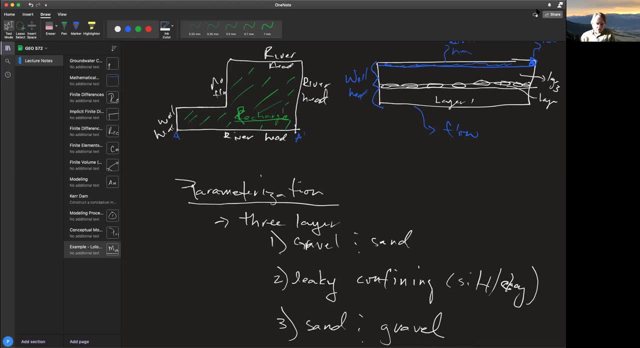 we're gonna want to make sure that we think about: well, what if I don't have those boundaries right? What would happen? And so that's where numerical models come in such handy. We can start playing with them. Well, I could change the amount of boundaries. 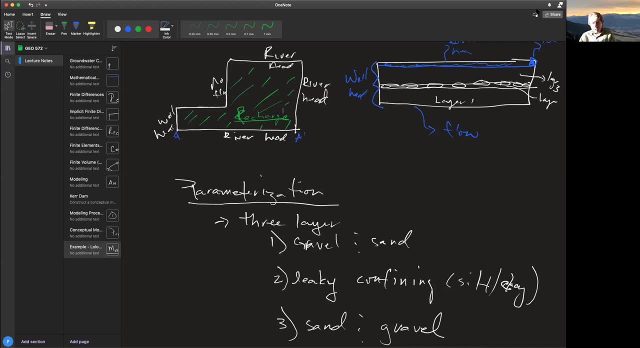 Yeah, I allow some blocks out of the mountain block. That's reasonable. Maybe I'd say, hey, whether it's not a no-flow boundary. I've already made And I say: what's some other way to derive a boundary between them? 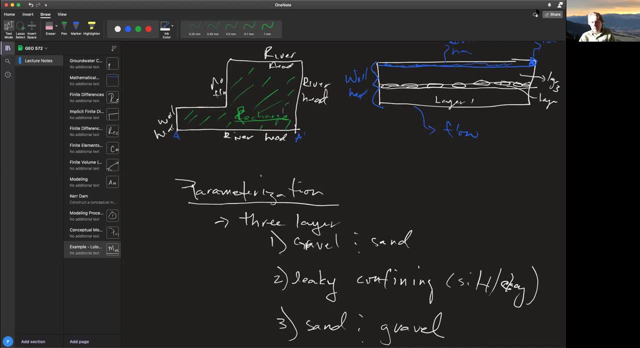 I can vary the different kinds of layers. I can vary how I look at parameterizing surface hydraulic conductivity. They don't be layers at all And I just do a random generation and play with it every once in a while. All of these things are things that I can play with. 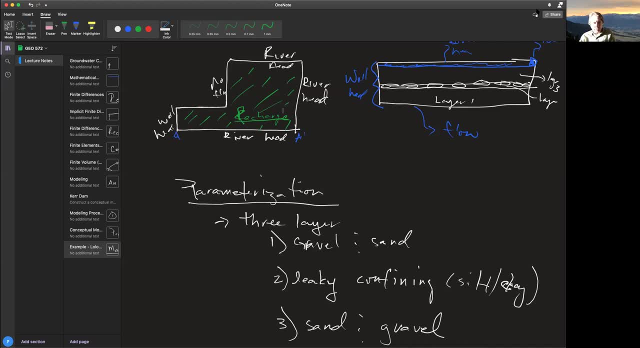 if I remember what my assumptions are and how they build in that certainty. Okay, so I hope this gives you just some example of how we might go about building a perceptual model, But I want you to remember that it's not right, right. 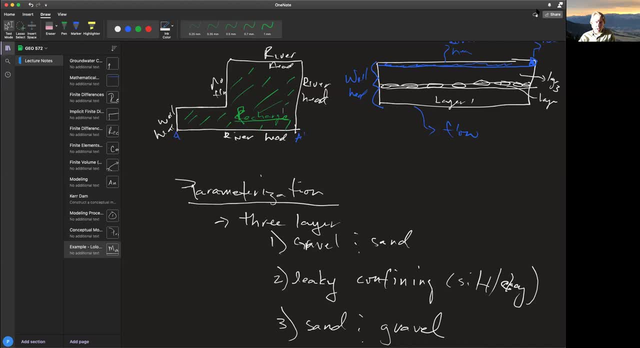 It's not wrong either, as long as we remember where we simplified things and how we might interchange them when we're looking at making corrections. All right, we'll call that for the day. Have a good evening and I'll see you tomorrow. Have a good one, bye.